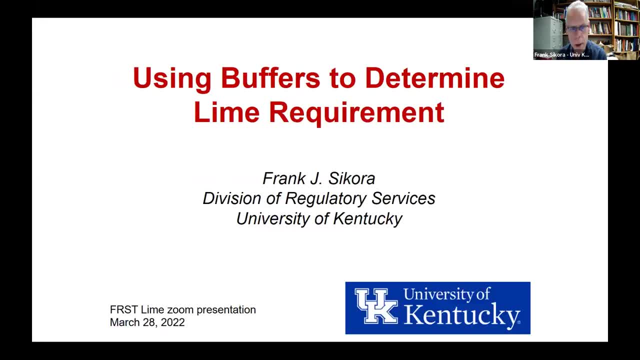 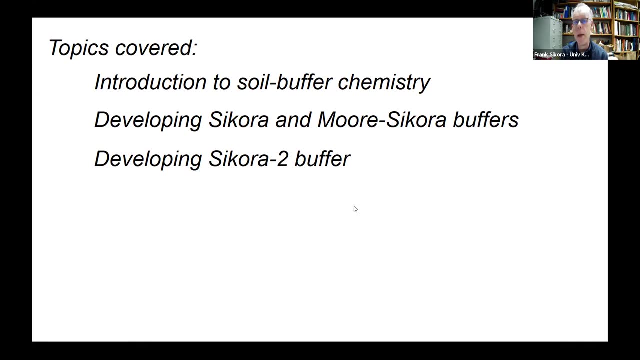 But I'll just start off with this title slide. here You all see the title slide in full. Yeah, okay, Okay. So what I'm going to be covering here are: introduction to soil buffer chemistry, developing the Sikora and more Sikora buffers, and developing the Sikora II buffer. 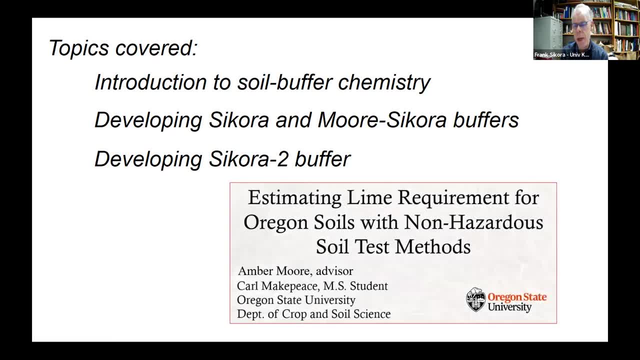 I also want to thank Amber Moore and Carl Makepeace at Oregon State University because they conducted some recent studies just in the last couple years that really added some more information to the Sikora II buffer that I'll discuss a little later. So I'm going to go ahead and get started. 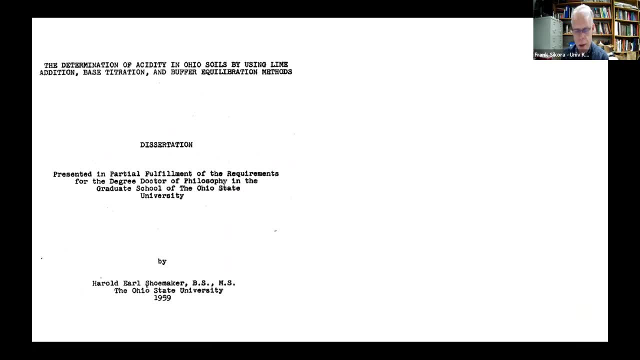 Well, when I first started into trying to understand buffers and study the topic, one graph that I thought was really important to understand it was found in Shoemaker's dissertation, And Shoemaker is the S in SMP buffer. You don't find this graph very much in the literature. 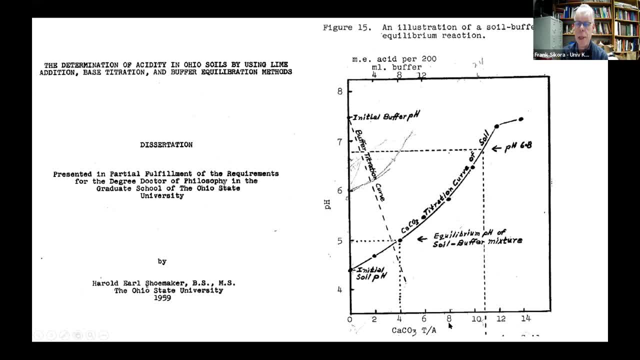 but I found it in his thesis. So he's trying to understand the S in SMP buffer and it's just this complicated graph here and i, i'm not. i'm. i'm going to talk about some of these lines later, but what i want to focus on now is just this line right here which represents: 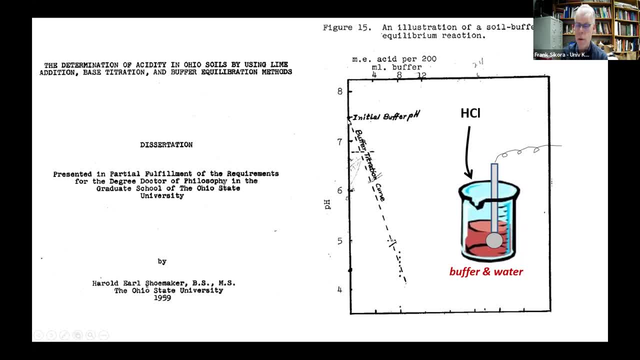 the titration of just the buffer. no soil, just the buffer and water in a beaker and you add acid to it. you're going to start off with some initial ph of the buffer and with increased amount of acid the ph would decrease. so you're looking at the titration curve of just the buffer. 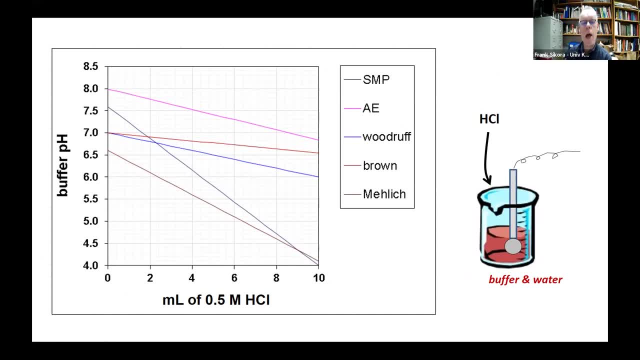 this is a graph of several buffers that are out there. with respect to that titration curve of adding acid to the buffer uh, buffer and water is mixed together. mixed together in the volume of water and buffer uh is the volumes that are used in the method of testing first soil ph with water and then adding. 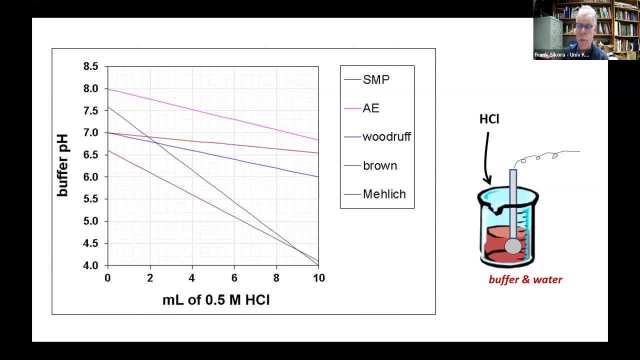 a certain volume of buffer. so you have that certain combination of buffer water, you add acid and you're going to get a decrease in ph. so you see, all these buffers we have out there, they have all different uh buffering capacities with respect to the ph, uh with addition of acid. 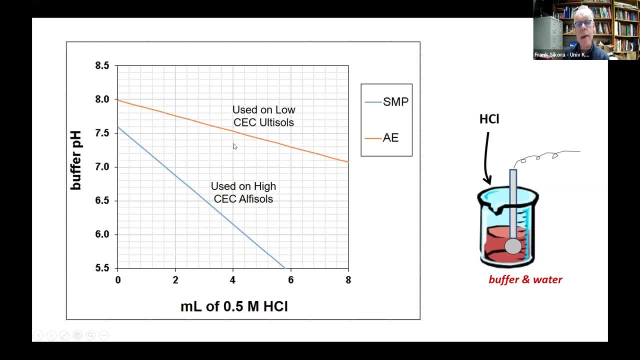 the adams evans buffer is an orange here and that's ae and that is a really strong buffer. you, when you add acid, the ph does not decrease that much. the ph begins at eight and it decreases uh moderately with increased acid. uh, the smp buffer, uh is a weaker buffer. the. 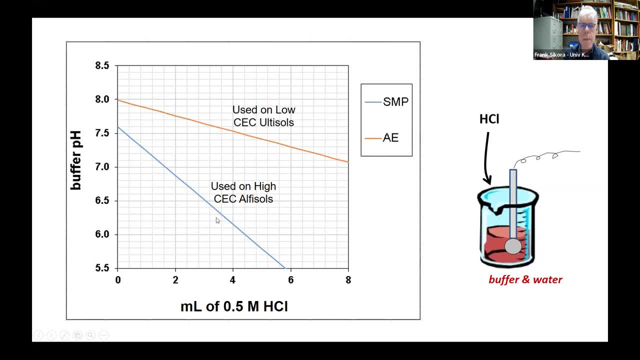 ph decreases more drastically with uh increase in acid. the adams evans that i'm sure everybody's aware is used on uh altisols, low cec soils. it was developed in alabama. the smp buffer was developed in ohio on higher cec soils such as observed in alpha cells. you'll often hear in the literature. that the buffer chemistry is well suited to the alpha solist, which is used in the Reality solid. that the buffer chemistry is well suited to the weight of the alpha solist, which is used in the Reality solid. the buffer chemistry is well suited to the weight of the high temperature cores. 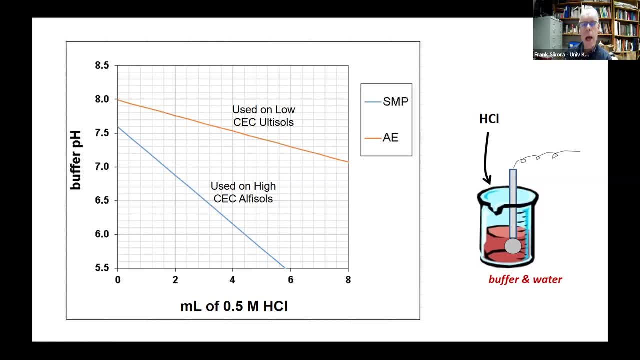 suited to a particular type of soil? uh, i don't believe that to be the case. i think these different buffers are appropriate for different types of soils because they are calibrated. they were cali. the buffer ph was calibrated to lime recommendations for those particular set of soils. 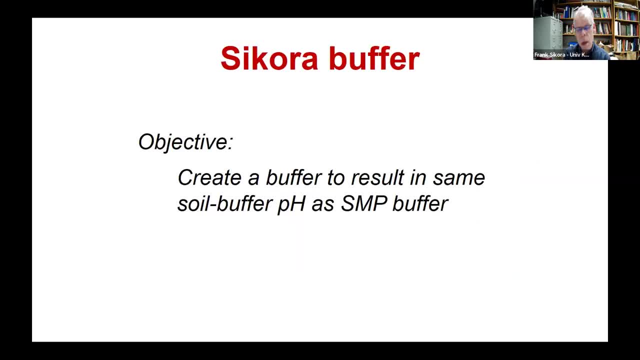 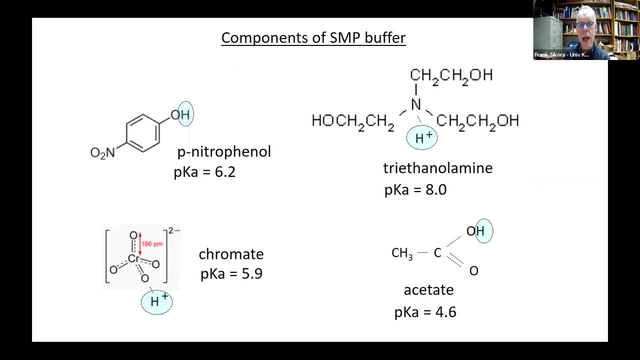 so that's it on the introduction of the chemistry uh. in creating the sakura buffer, the objective was to create a buffer to result in the same soil buffer ph as smp buffer, and the main reason for that was to get rid of the hazardous chemicals para, nitro, phenol and chromate in the smp buffer. 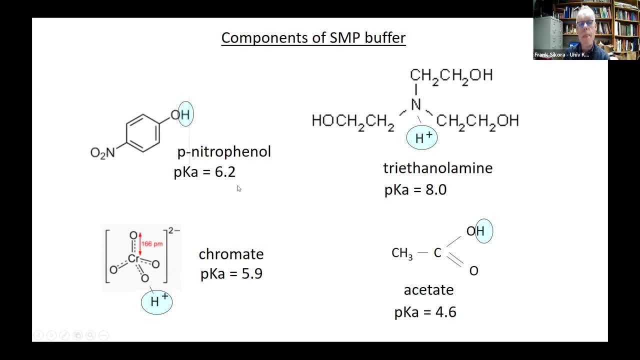 these are chemicals that are used to create the buffer ph and they're used to create the chemicals that could not, should not, be dumped down the sink. they had to be disposed of a certain way. so, uh, not only myself but others have been looking at these buffers to remove these hazardous 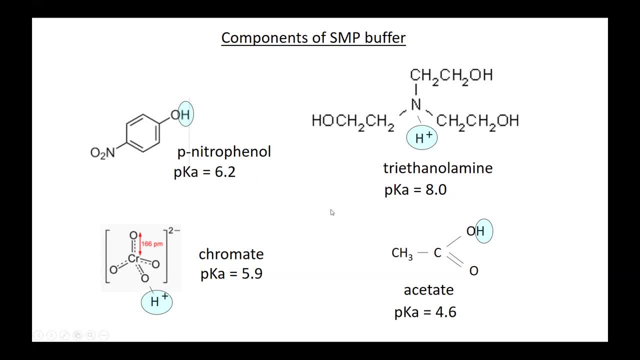 chemicals. uh, one aspect of all these buffers that i showed earlier is they have all combination of different acids and bases in the buffer and this combination of these different acids and bases results in the linear decrease in ph as you add acid. that is very important for all these buffers. you have to have linearity, a linear decrease in ph with the addition of acid. 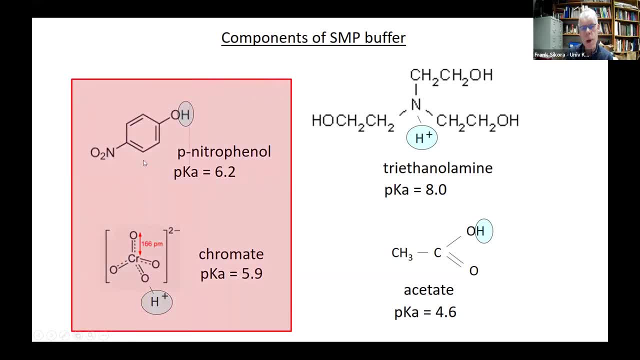 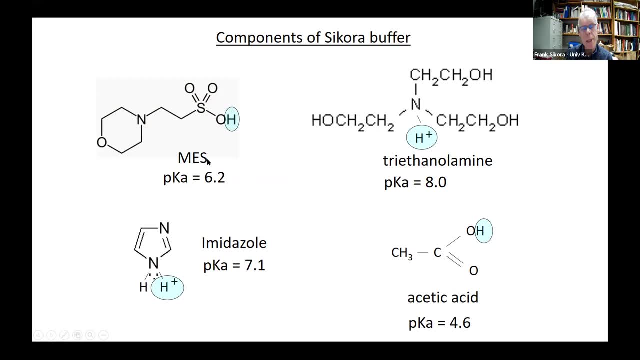 so with this work, we wanted to get rid of para, nitro, phenol and chromate, and it was replaced with the chemical abbreviated as mes and imidazole. and you see the pkas there. uh, i just played around with a lot of calculations, theoretical calculations, to determine what concentrations of these chemicals would be appropriate. 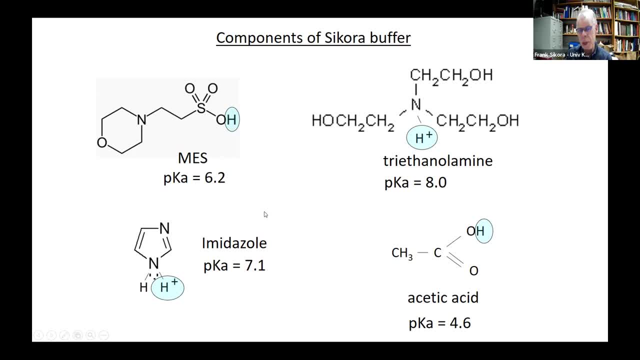 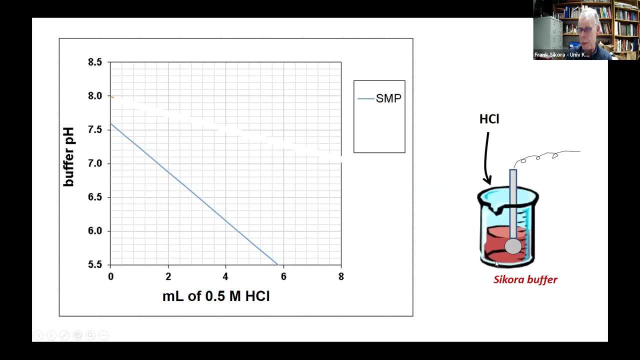 to result in a linear decrease. that was exactly the same as the smp buffer, uh. so again, i didn't work with any soil at all in this project. it was just looking at a solution of a water and buffer and putting the acid to it. uh, you have a decrease in the ph with the addition of acid to the smp. 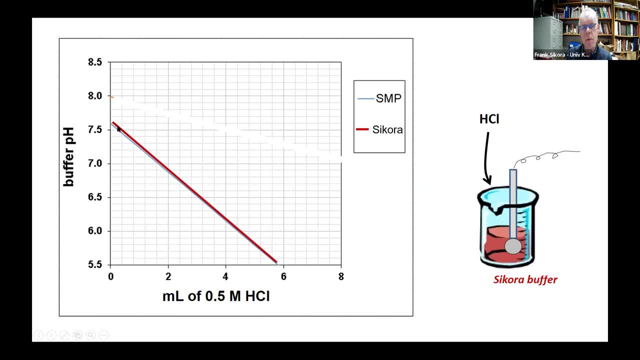 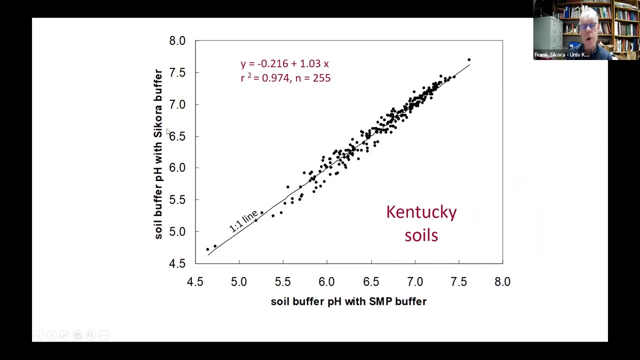 buffer, creating the sakura buffer. i mimic that with the same titration curve, uh with those replacement chemicals. well, this graph shows a comparison of using the sakura buffer with uh uh uh. comparing the sakura buffer and the uh pH with the SMP buffer pH by adding 10 mils of buffer to 10 cubic centimeters of soil. 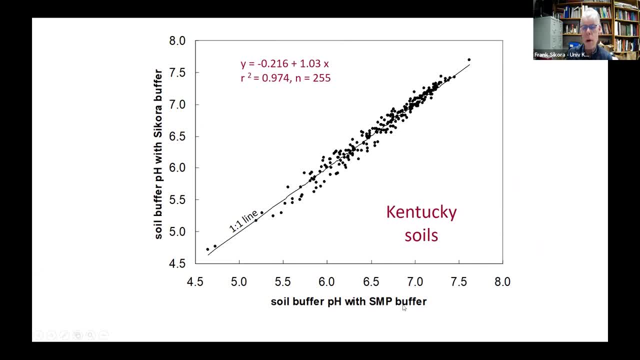 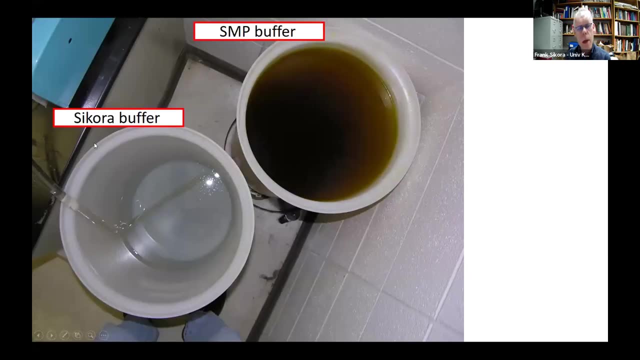 and then adding 10 mils of the buffer, either Sikora or SMP buffer. There was a good agreement between the two and the one-to-one line is here and you see the scatter points around the one-to-one line in a high R squared. This is a photograph of the Sikora buffer on the left. 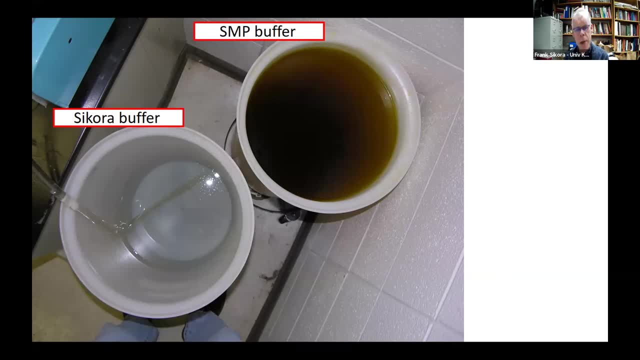 and the SMP buffer on the right. When I show this slide, I like to tell people I was really proud to create a buffer that did not look like piss. The SMP buffer just looks toxic. It looks nasty. The Sikora buffer looks clean and fresh. 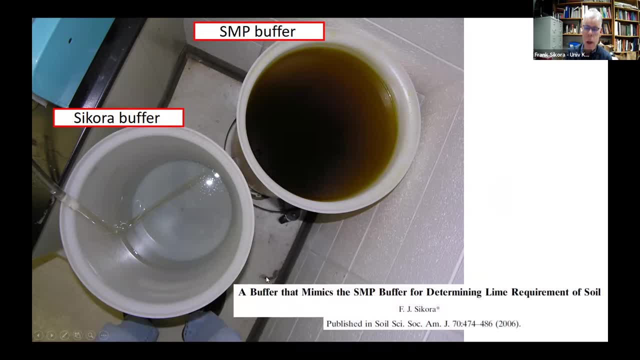 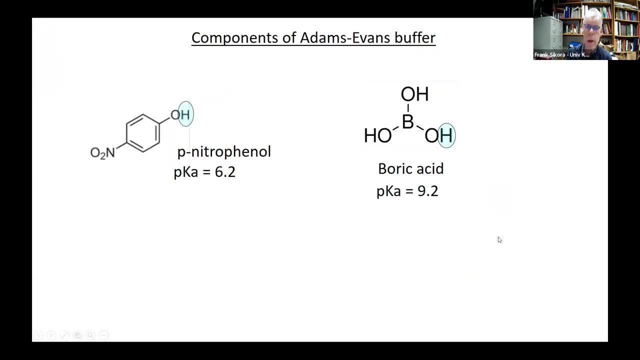 The publication on creating the Sikora buffer is shown here, if anybody wanted a reference to that. Well, when I presented this at the SIRS 6 meetings at Cathy Moore at Clemson, she said: well, can we do the same thing with Adam's Evans? Adam's Evans has perinitropenol in it, Could we? 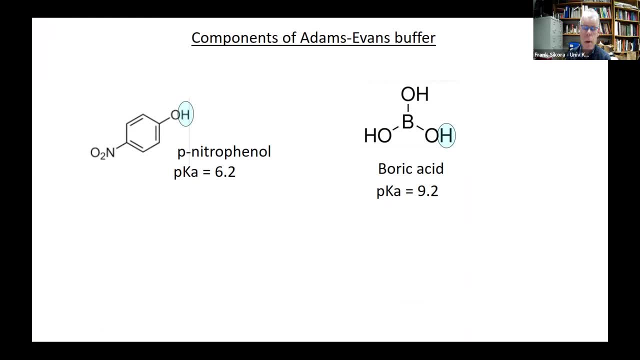 replace that with another chemical to have the same acid titration and result: the same buffer pH. So I said, yeah, we'll try it and we worked on that. We got rid of perinitropenol in the Adam's Evans buffer. We replaced that with MES and MOPS. With this buffer we had such a MES, we needed MOPS. 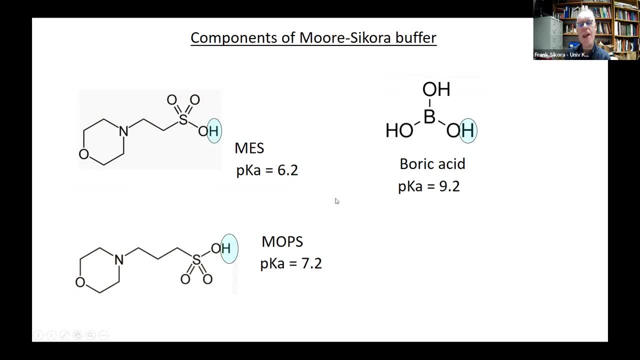 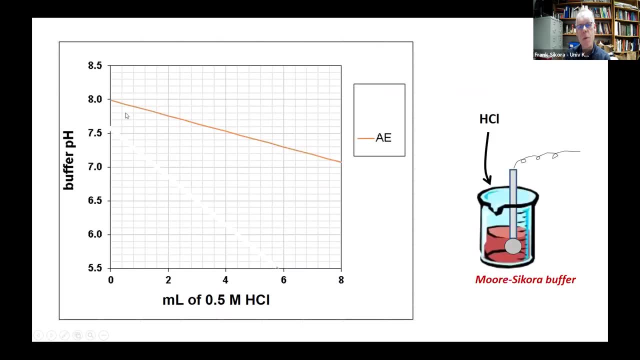 You see, I mean that was a joke there- But the combination of these different acids was played around with to make sure that we had a linear decrease in the pH with increased acid. This is the titration curve of the Adams Evans buffer and this is the titration curve of the Moore Sikora buffer. So we just had the same. 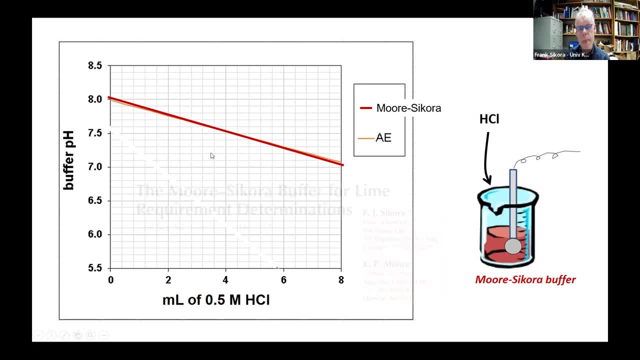 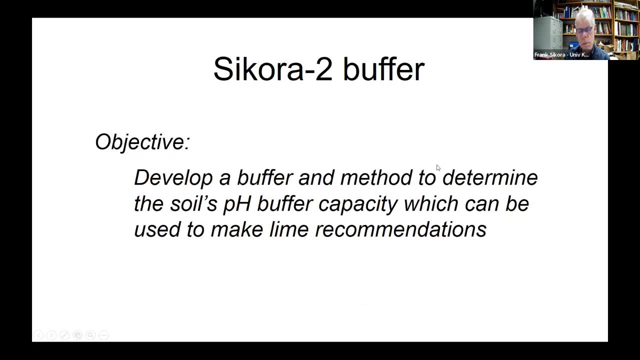 titration with respect to adding acid. The reference to that work is shown here. The work I showed so far was pretty much a chemistry project, a laboratory project. It didn't really evaluate or look at lime recommendations. The objective was just to create a buffer that would give the same buffer pH value as the buffers that were being replaced. 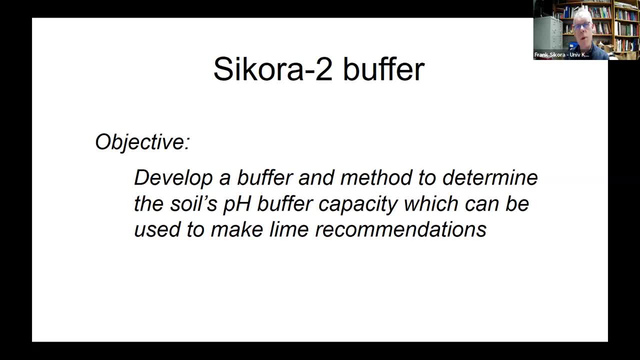 The Sikora II buffer, looked at it a little bit more with respect to the lime recommendation that we would make based on those buffer results, And the objective of this work was to develop a buffer and a method to determine the Sol's pH buffer capacity which can be used to make lime recommendations. 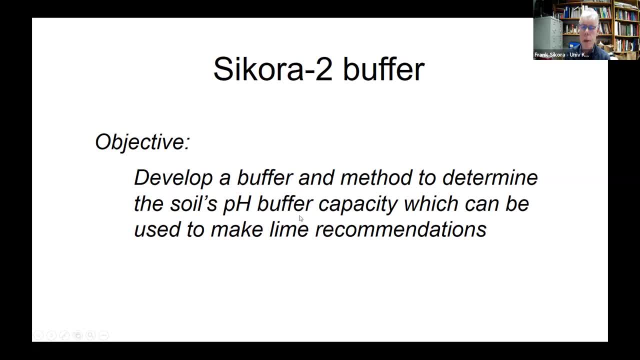 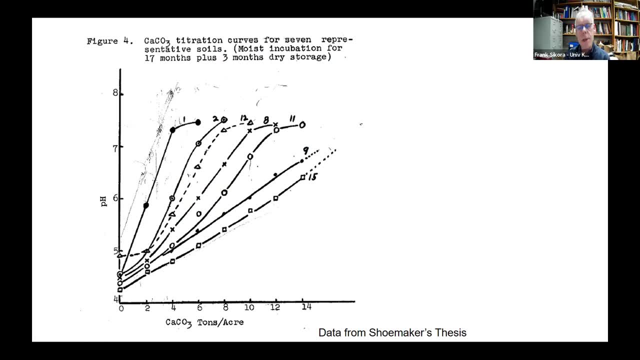 So the Sol's pH buffer capacity are the important words here in this objective. And this is a graph from Shoemaker's thesis and it's just showing typical lime response curves with the addition of calcium carbonate to soil- We're all familiar with this- You increase calcium carbonate. 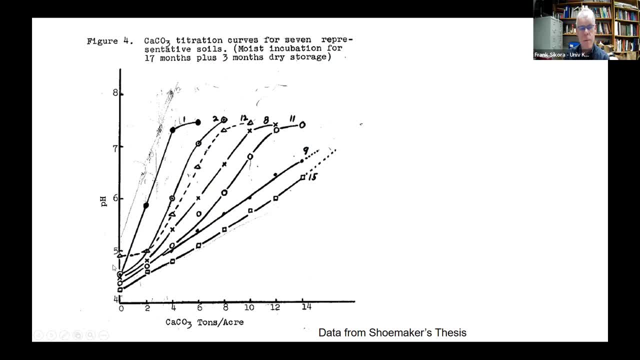 you're going to get an increase in pH for soils that are very acid. With these lime response curves and developing a method, it's very important to know what the slope is. That's the important parameter. I think we should seek to make lime recommendations. 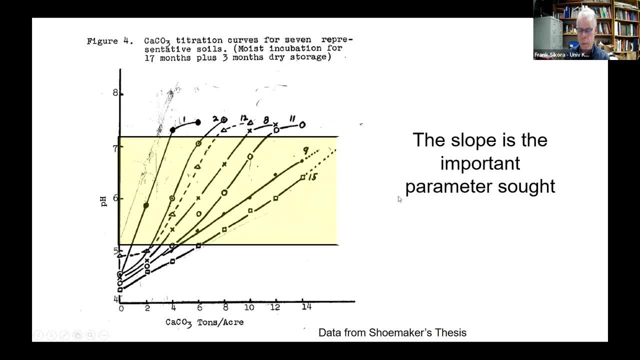 And this was the objective not only in the work for the Sikora II buffer, but also the work that David Kissel did with the single-addition calcium hydroxide method in Georgia. The objective was to determine what the slope is for the lime response curve. 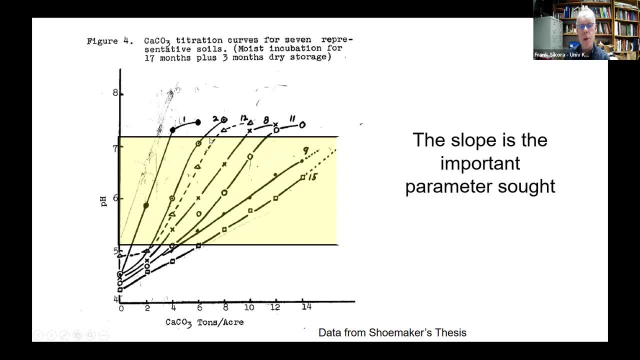 Because between a pH of about 5.2 to 7.2, it's pretty linear. So if you determine the slope of the response in this pH range, it has a lot of advantages. You can determine a lime requirement to any pH. 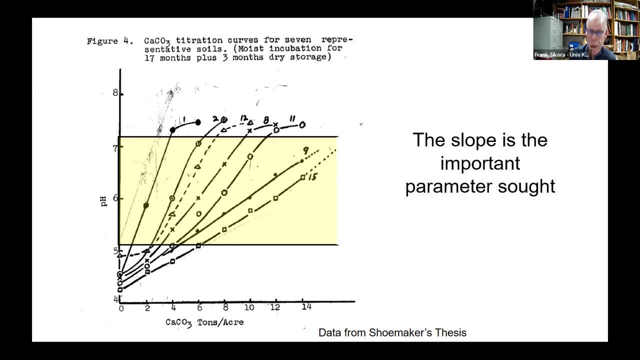 You don't need separate tables or equations for different pH targets. You could use algebra to calculate what lime is needed to reach a certain pH, And it's also a method that would be suitable across a lot of different pH targets. And it's also a method that would be suitable across a lot of different pH targets. 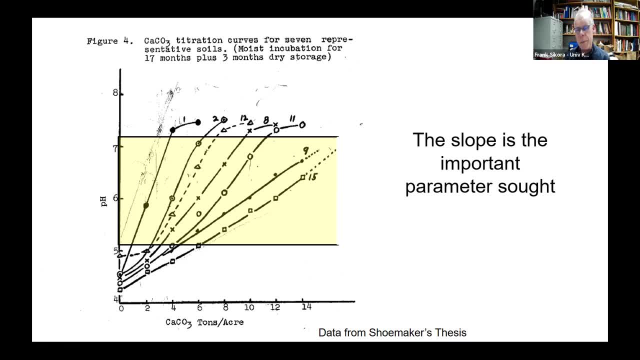 And it's also a method that would be suitable across a widely-differing salt types — low CEC to high CEC salts, And you could also possibly use it to predict how much acid to add to decrease pH. So there's a lot of power, I think, in knowing what the slope is. 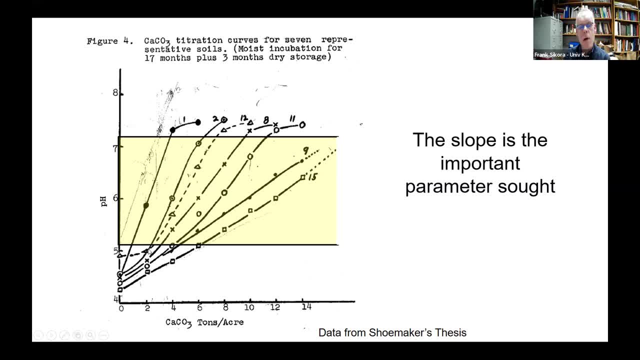 for the lime response curve, But it's also a method that would be suitable across a widely-differing salt type buffering the pH, And if soils are very high in pH, you have calcium carbonate buffering the pH. So knowing the slope is only going to be instructive between pH 5.2 and 7.2.. 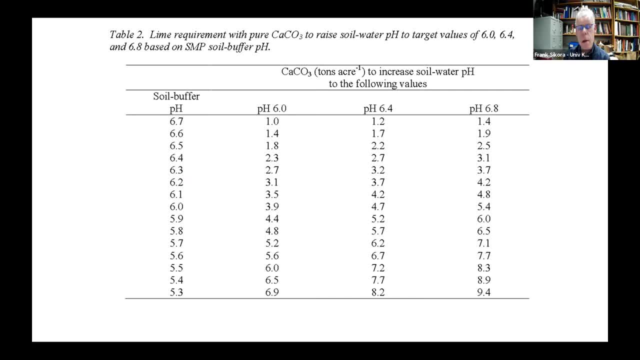 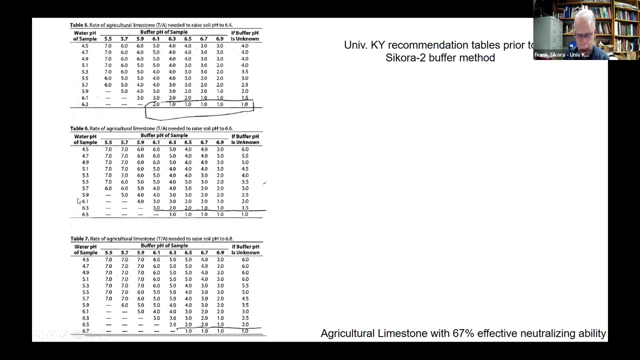 This is a typical calibration table for SMP buffer showing how much lime to recommend the different target pHs with respect to what the soil buffer pH is. So for one target pH it's only looking at what the soil buffer pH is to make a recommendation on how much lime there is. When I came to Kentucky in 1998 and I looked at our 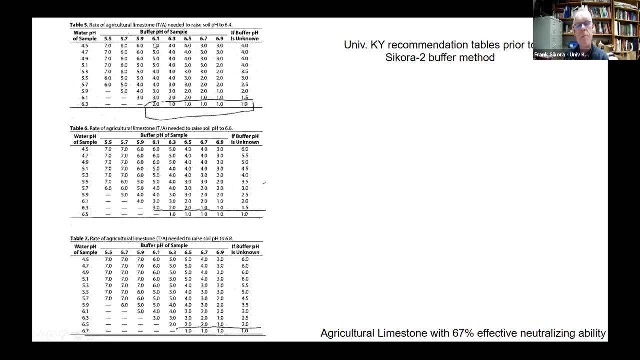 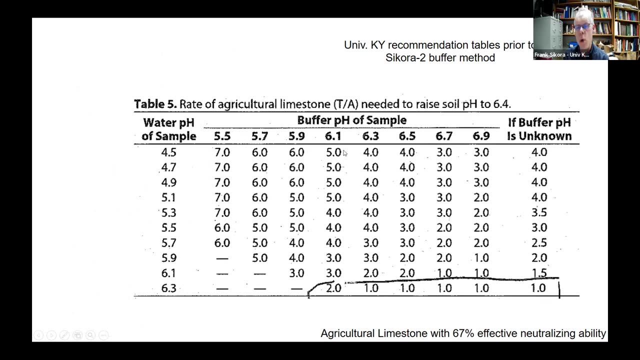 lime recommendation table. I saw that they were using the SMP buffer and the water pH of the sample together to make a lime recommendation And I'm showing just one of those tables here. The previous slide showed a table for each target pH. I'm showing here the table just for the target pH of 6.4.. And you know I asked why. 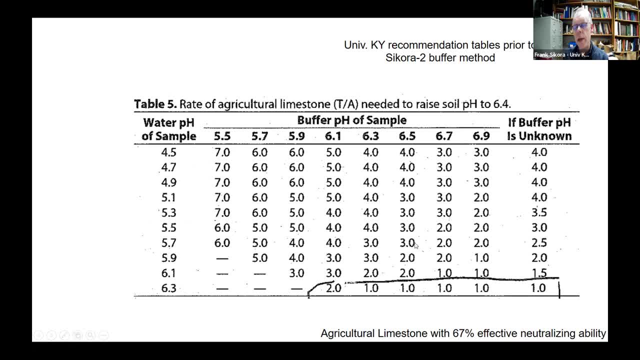 are you straying from the initial SMP calibration tables? And they did not have any. the soil specialist didn't have. all they had was empirical data, a best guess at what these recommendations should be. And their argument made sense If you had a buffer pH of 6.5 and you looked at just a previous 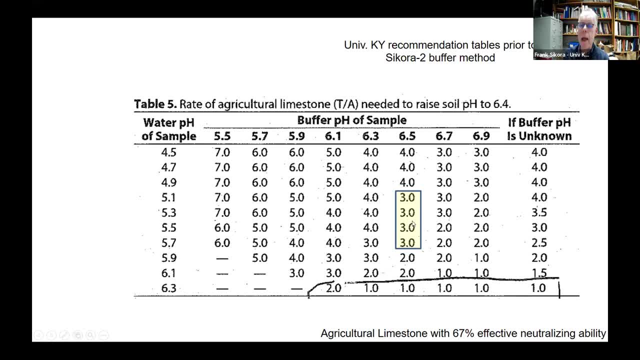 recommendation table. looking at just buffer pH, you might have a recommendation of three tons per acre, But if you're starting off with a pH that is really low, it would make sense that you should apply more lime. And if you your pH is higher, with the same buffer pH of 6.5, you should have 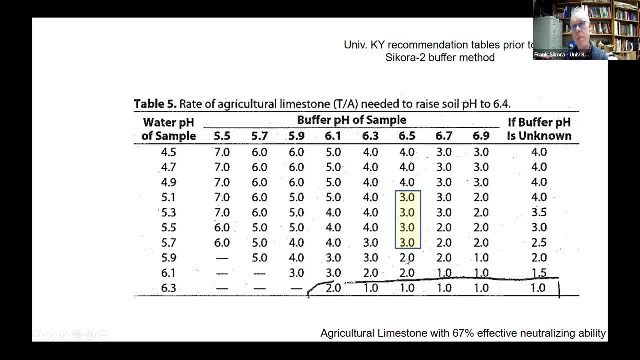 less lime being applied, So that made sense from an intuitive point of view. My uh goal was to develop an equation that could predict this, that could use a lime response curve that could be evaluated from buffer pH to predict these values we had in our recommendation table. 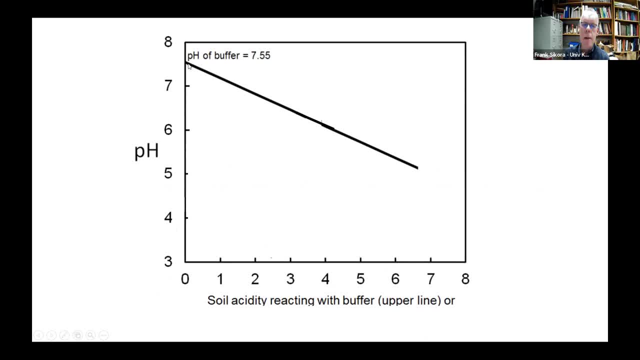 So to do that, I went back to thinking about this titration curve of the buffer with addition of acid And you have a certain soil buffer pH that you might get from adding the buffer to the soil, And here it's a soil buffer pH of 6.5. 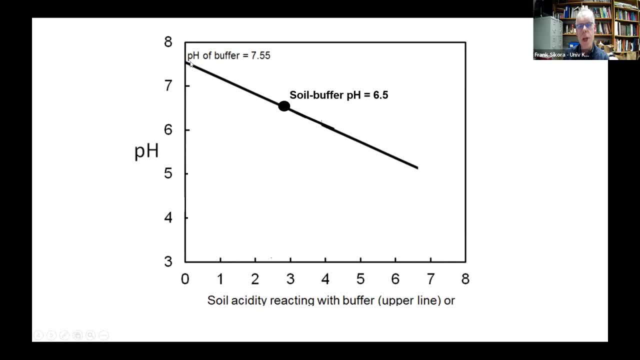 So it would take so much acid to decrease the pH of the buffer from seven and a half to 6.5.. You could also overlay on this graph the amount of alkalinity from the buffer that is required to increase the soil我說 pH to 7.5, 6.5.. of pH from 세 thì dit từie 마 до 6, 5, 5 많as Acele alphabet Bobbitt trusting. following the, that D into 7.5 was at 379 F, 6.5, 9.4 and 28.7.. 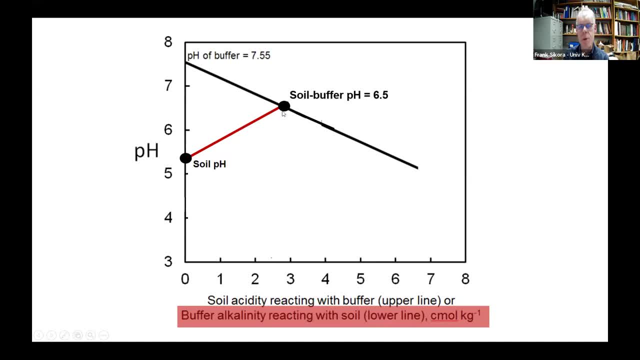 soil pH, from some initial pH here about 5.2, to this soil buffer pH of 6.5.. So this red line is a lime response curve. It's the pH of the soil increasing with respect to the with the addition of the alkalinity from the buffer. 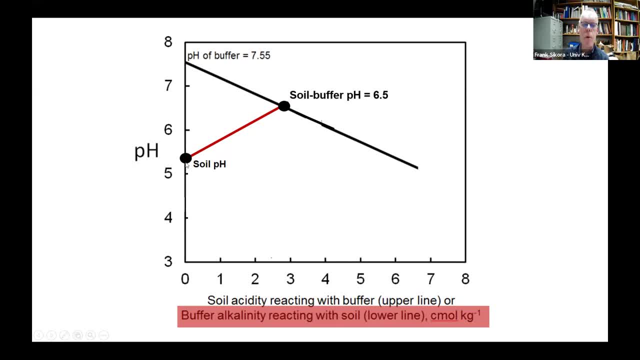 So if you take that concept from the previous calibration table that if you're in the middle of a soil pH you're going to recommend so much lime to get to the target pH value, But if the pH is higher you would require less lime to get to that target pH. But if the pH is 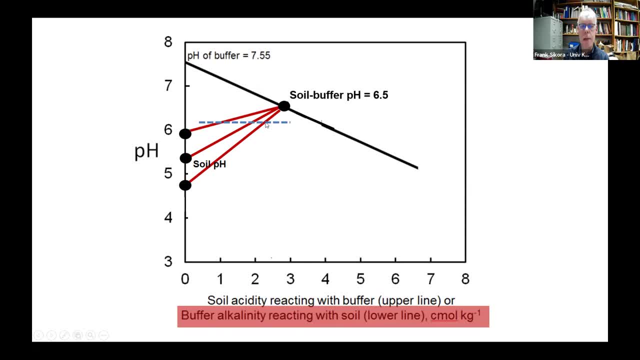 lower, you would require more lime to get to that target pH. So this is just graphically trying to make sense of what was in the table: That the lime recommendation should not only be based on the soil buffer pH but it should also be based on the initial soil pH. 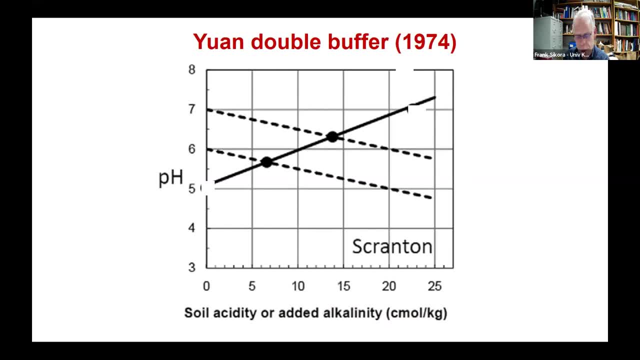 In this concept of using two pH values to determine what that lime response curve is is what was used in the double buffer method that Juan developed in 1974.. I just show this here to indicate that it wasn't a new technique that I was using on using two buffer or two pHs. 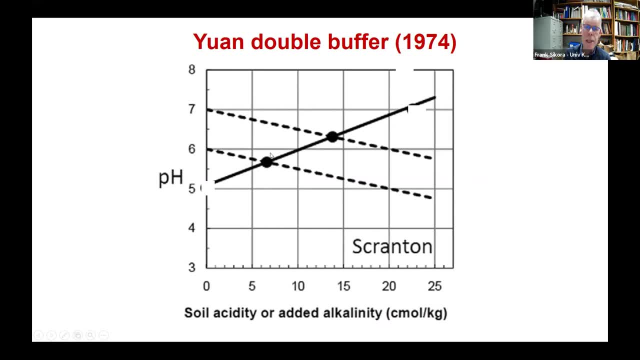 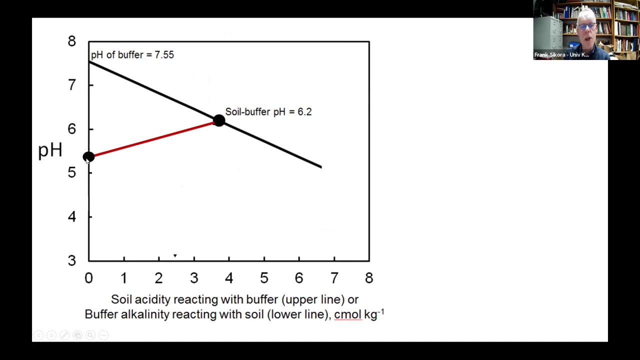 Because the double buffer methods also use that same concept. The difference I was interjecting in the study was having one of those pH measurements just being the initial soil pH, not a pH from a second buffer. So we go back to this curve here where we have lime response curve, with the initial pH. 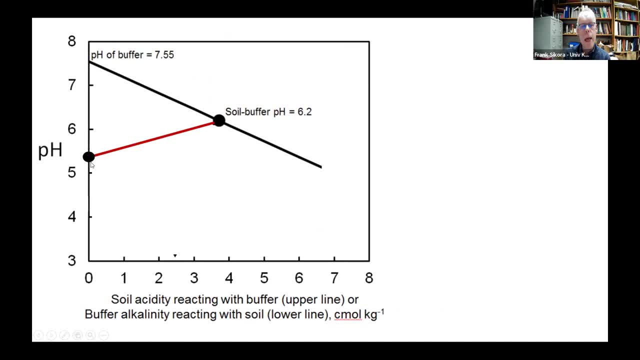 and then the soil buffer ph and i. i showed just a a general graph of that a couple slides ago. but when you start thinking about what the salt concentration is with an initial soil water ph and the soil buffer ph, i started to realize that we were- i was comparing apples with oranges. 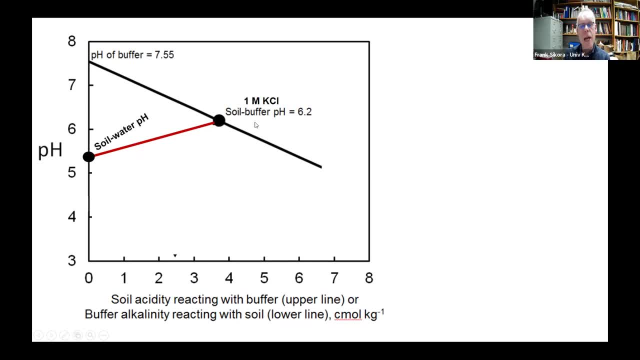 because the soil buffer ph has the uh salt concentration of one molar potassium chloride. so water ph, you know it might be 0.01 molar ionic strength. so that's why i introduced the one molar potassium chloride salt ph to get the ionic strength of that. 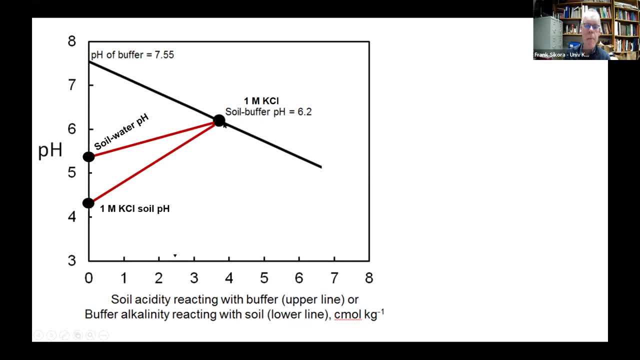 initial salt ph to be the same as the initial ionic strength of the ionic strength in the soil buffer, ph, so that apples could be compared with apples and a adequate line response curve could be drawn between those two points, the target ph. if we're looking at this line response curve, the target ph, 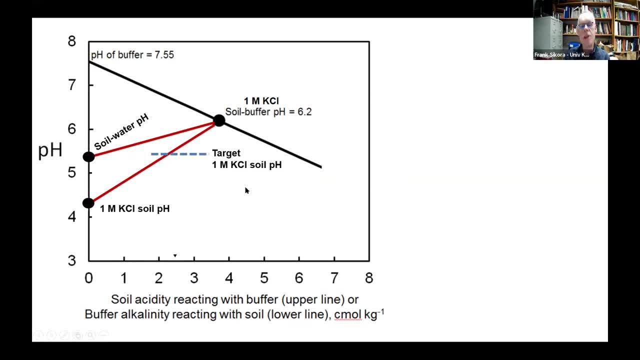 would need to be what the ph is to raise it, what, what alignments needed to raise the ph? uh to a one molar potassium chloride salt ph or target and the working with all this, you have to get what the relationship is between your soil water ph and one molar potassium chloride salt ph. it's approximately one, so that's why you see this. 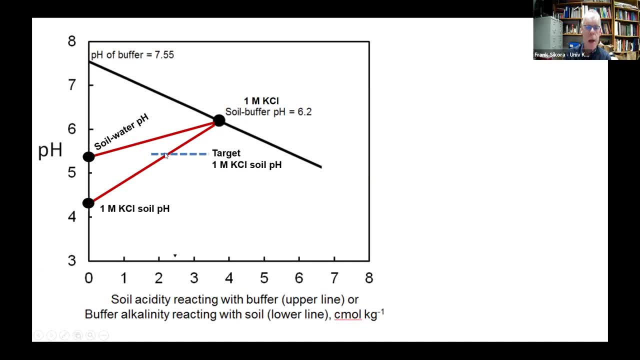 decrease in one ph unit and uh. this target ph unit 5.4 is approximately equivalent to 6.4 or a salt water ph. so the figures on the right are showing what the difference is between a sakura buffer and a sakura 2 buffer. in the sakura buffer you see the salt concentration in this buffer. 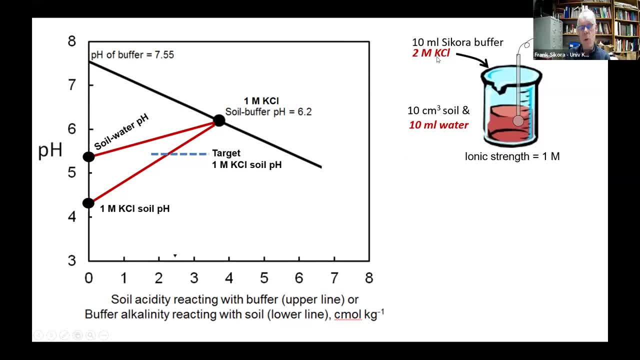 as it was in the s? p buffer, is two molar potassium chloride and that high salt is in there to exchange uh, to release exchangeable acidity in aluminum from the soil, so it could be neutralized by the bases in the buffer. so when you're adding 10 mils of two molar potassium chloride solution to 10 mils of 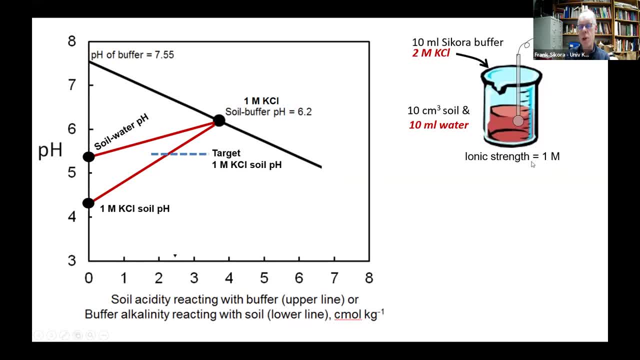 water. the final ion strength of that solution is one molar. well, if we're going to start off with a one molar potassium chloride salt ph. as the initial ph, the concentration of potassium chloride had to be reduced in the in the buffer. so that's what the sakura 2 buffer is. it has half the potassium chloride concentration- one molar. 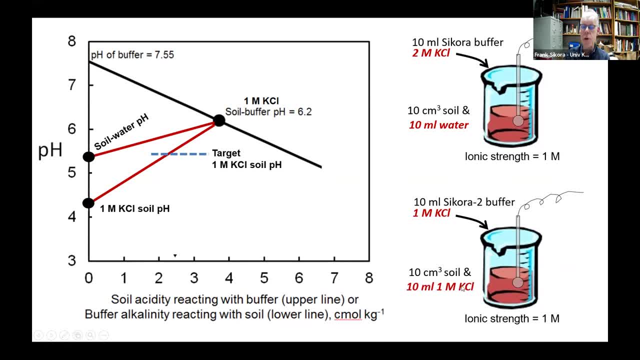 potassium chloride. so when it's added to the solution, measuring the initial ph, the ionic strength is one molar. so that's. the only difference between these two buffers is the concentration of potassium chloride. the acids and bases, their concentrations are the same and the ph that is obtained from these two methods are the same. 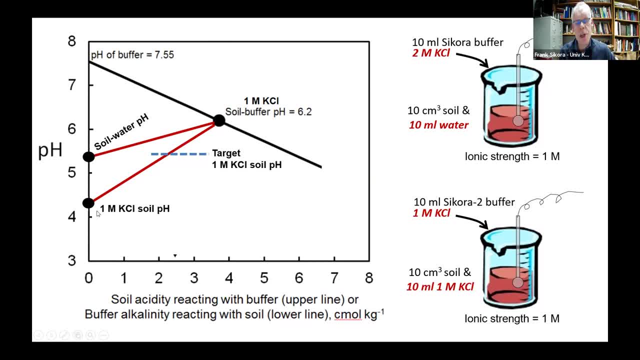 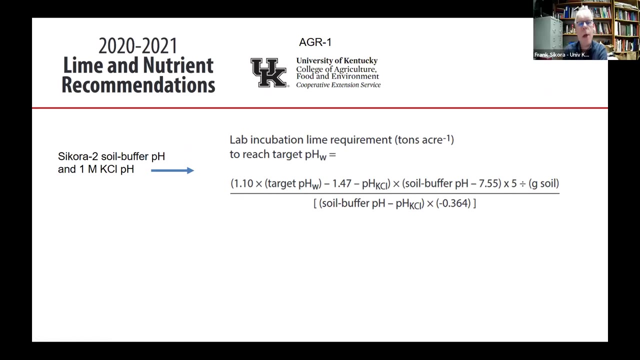 so that was the reason the high salt concentration was introduced in this method and it had a side side benefit of getting a soft ph. of all the benefits that were discussed with you a month ago when we looked at the advantages, all right, all right, sounds good. okay. so this is the equation to calculate what the lime requirement should be in tons per acre. 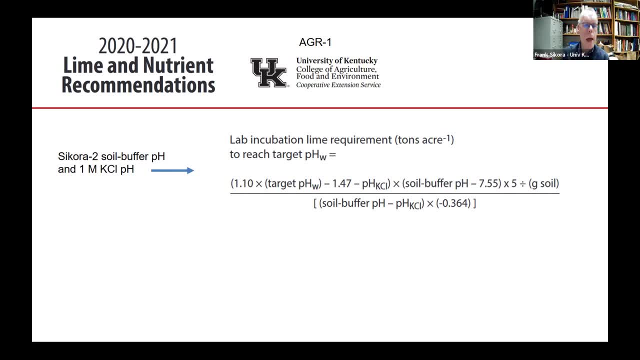 to reach a target water ph with a score tube buffer and initial ph one molar potassium chloride just using algebra and the line response curve. What's highlighted in yellow here is the relationship between water pH and potassium chloride soil pH, so that we can plug in a 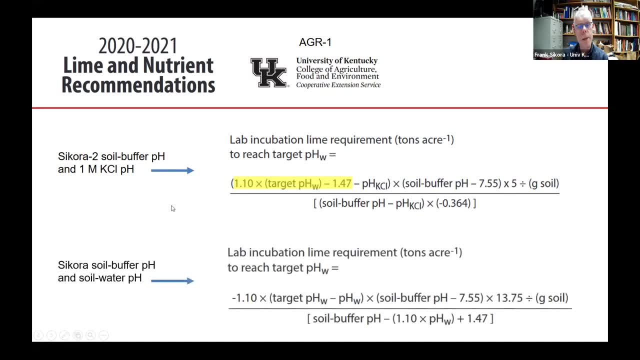 target water pH. This method could also be used with a sakura soil buffer pH and soil water pH, where you have the relationship here, replacing the the initial pH of potassium chloride with initial pH and water. knowing what the relationship is between KCl pH and water pH. 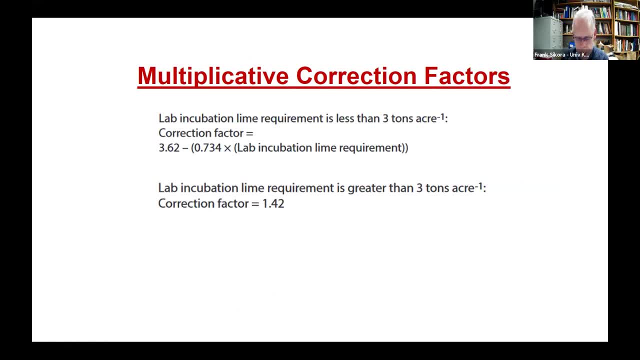 Well, much to my dismay this, the formulas in the previous graph calculating lime requirement did not produce a value that we had in our recommendations tables of UK, and what I've observed is I needed a multiplicative correction factor to multiply the equation line requirement by a correction factor. 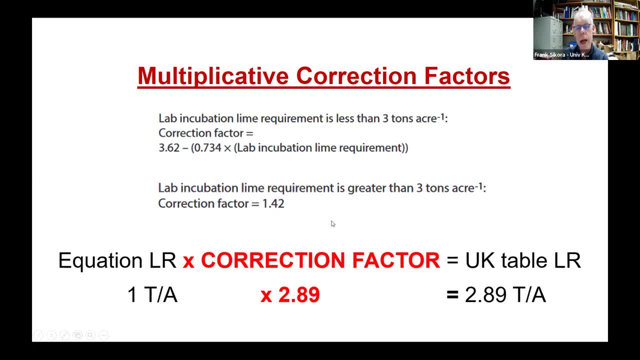 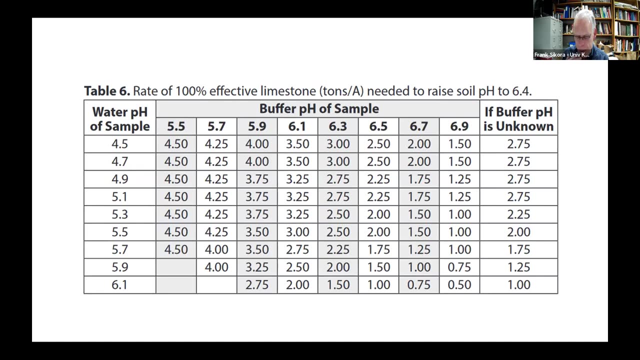 to get to values in the table, and these, these are the equations to obtain those correction factors. The question is: how can we compute the value of the equation, And that is one thing that I wish I had more time to study. I did not do any lab incubation. 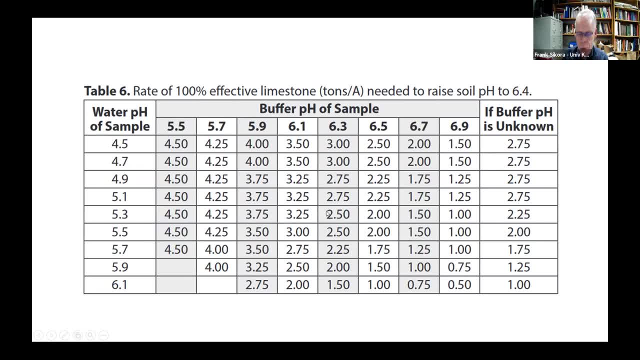 experiments to verify this. All I was doing was trying to get back to the values we had in our recommendation table so it could be calculated with one equation, factors uh. in our current recommendation table, uh shows a lime requirement a little differently here, because it's based on a hundred percent effective lime uh and it's uh rounded to the. 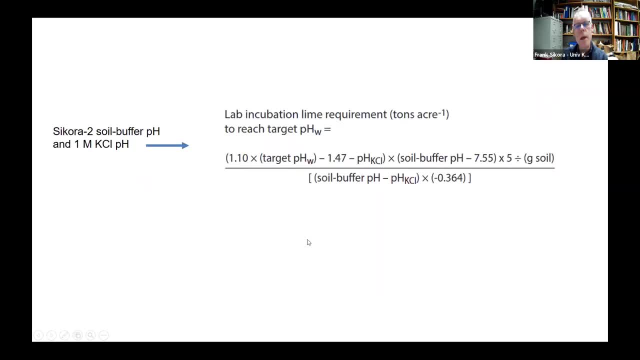 nearest quarter of the ton per acre. but i want to get back to this correction factor. uh, and when i created these equations and put them in our extension publication, i assumed that what we were painting was the lime requirement. that would be typical from a calcium carbonate lab incubation. so i i would say: lab incubation line requirement times the 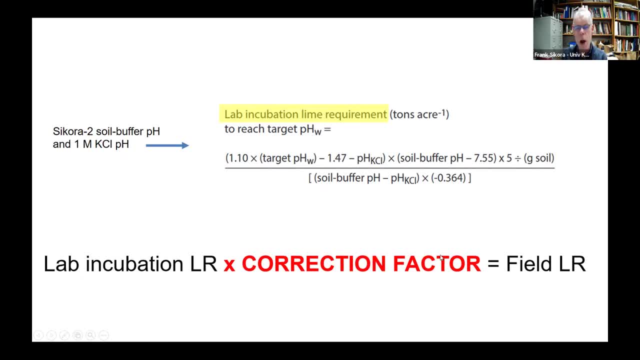 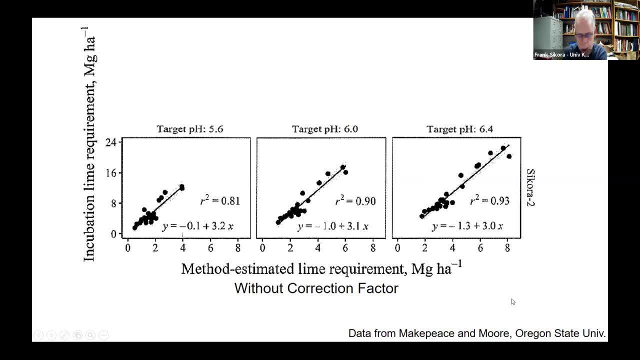 correction factor would equal some field line requirement and i thought we needed the correction factor to get from lab incubation to field lime requirements. well, the data from carl and moore at an oregon state and has proven this to be false. they they had calcium carbonate. 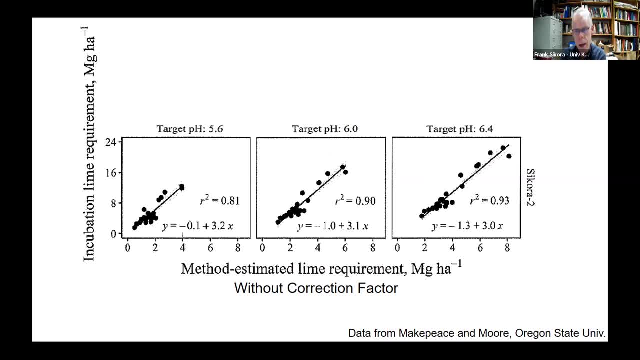 incubation study on oregon soils and they had. they did the socorro 2 method on these soils and the graph you're seeing here is the incubation line requirement from the calcium carbonate incubation versus the method estimated line requirement without the correction factor. so it's 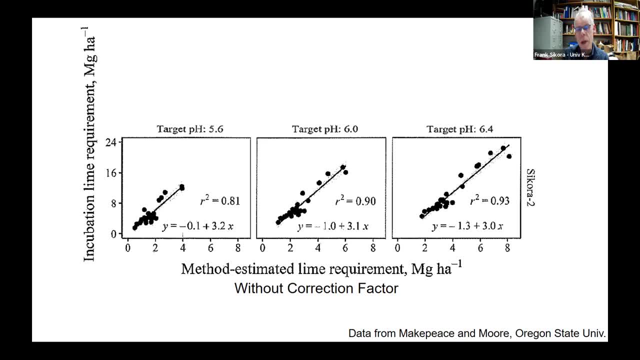 based on that uh formula i showed earlier, without correction factor. if that formula was actually calculating the incubation line requirement, the slope of these regressions should be one, but you're seeing the slope being about three. so the incubation line requirement is about three times that from the method estimated line requirement. 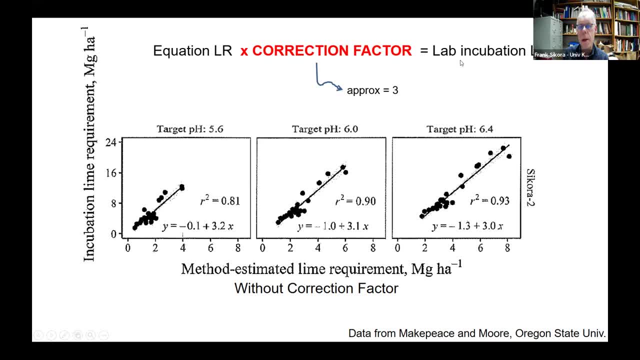 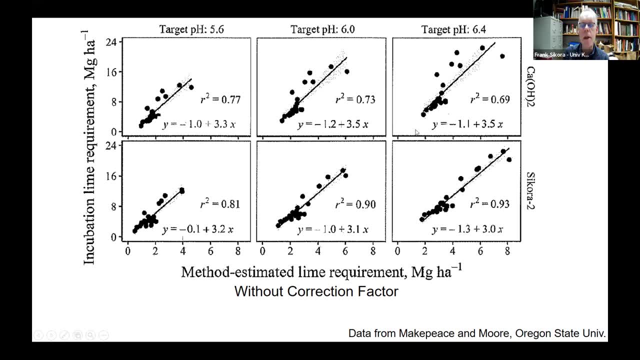 the equation line requirement times three is the lab incubation line. they also perform the single addition calcium hydroxide method and it was very striking that they had very similar slopes for about three. so it looks like about the same correction needed to be applied to the calcium. 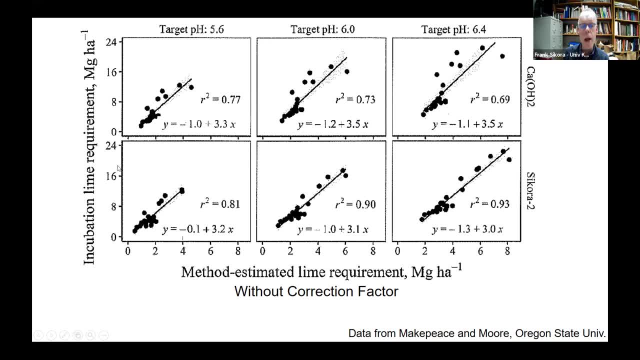 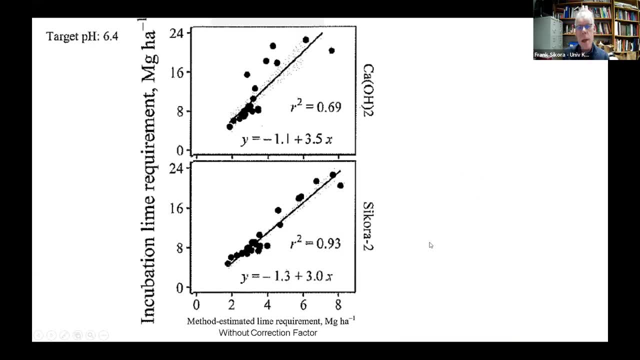 hydroxide method uh for comparing the incubation alarm requirement to the method estimated requirement. this graph is shown just showing the graphs for the calcium hydroxide core 2 method, with a target ph 6.4. and what i am overlaying on top of this are the correction factors that georgia uses with that. 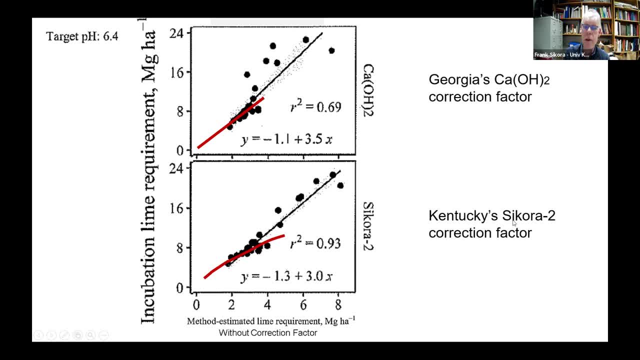 single calcium hydroxide method and the correction factor that we use for our method, and you see that it's very- i mean, it lies pretty much on top of the data they've observed and these correction factors do not go to higher line requirement because, uh, these, these high, these. 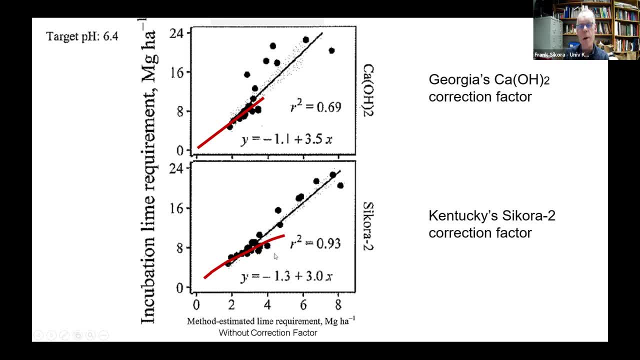 are extremely high line requirements, greater than five times per acre, and both georgia and kentucky pretty much top off max. a maximum line requirement is usually just five times per acre. so i mean i was very encouraged that this correction factor seems to be pretty consistent among the wide range of soils: the low cc soils in georgia, the higher 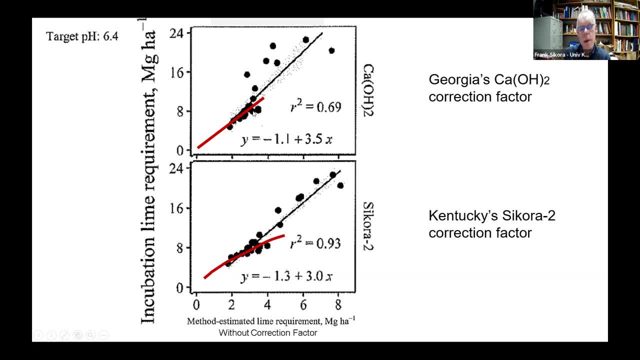 ones in kentucky and and the ones in oregon. so i mean, i i thought, if we had to introduce a correction factor, i was thinking, oh well, we'd have to calibrate this column, this correction factor, to different type of soils, but that may not be the case, so maybe one correction factor could be used. 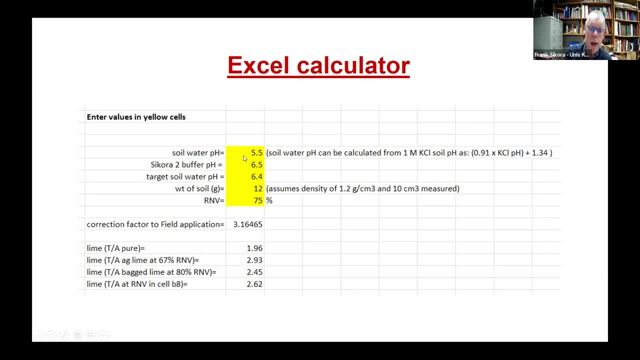 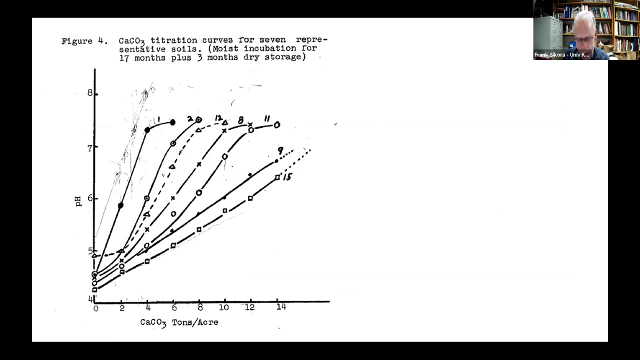 there is an excel calculator that i developed that we plug in any water ph buffer, ph, target ph to determine line requirements. i use this a lot when agents ask me to calculate live requirement of some ph. it's different than what we have in our tables, so i guess i this is my last slide that i want to end in. i want, i want to end with. 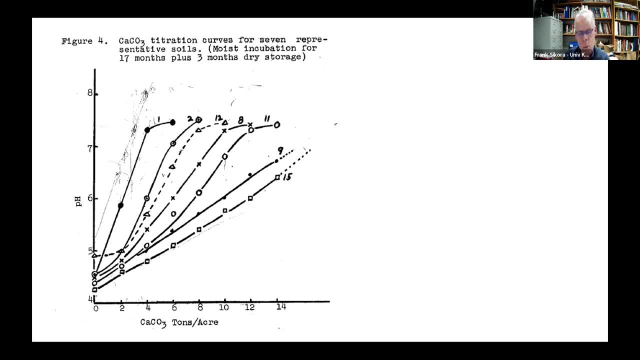 emphasizing again what i think is important is that it's not just about the water and the caloric important in this work of determining lime requirement, I think a very important parameter to be sought is the slope of this lime response curve, because once you know that, that's, that's. 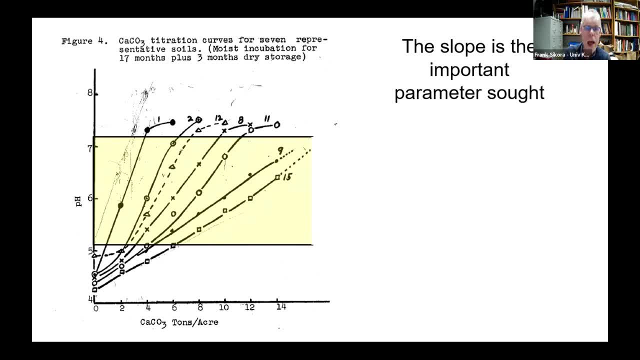 you. you have the answer if, if you have the parameter to calculate pH, a target lime required to any target pH. uh, it seemed it'd be suitable across a wide range of soils. so I'll end in a little bit of humor and say that I think this slope is the Holy Grail, the whole enchilada and 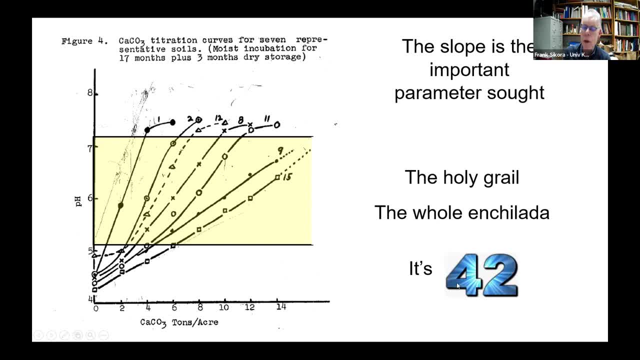 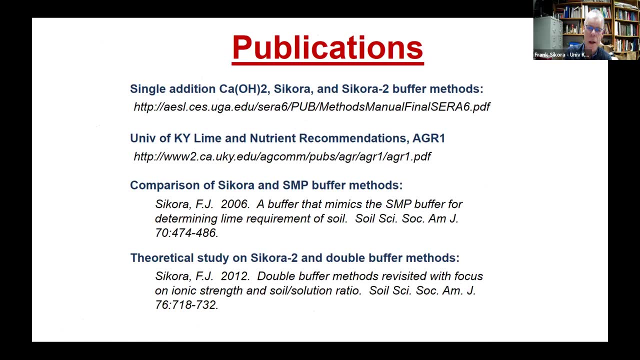 it's 42. and it if you have to seen or read the Hitchhiker's Guide to the Galaxy to know what 42 is. 42 is the answer to everything in the universe. so that is it. the publication has a list of references if you're interested in looking at it. 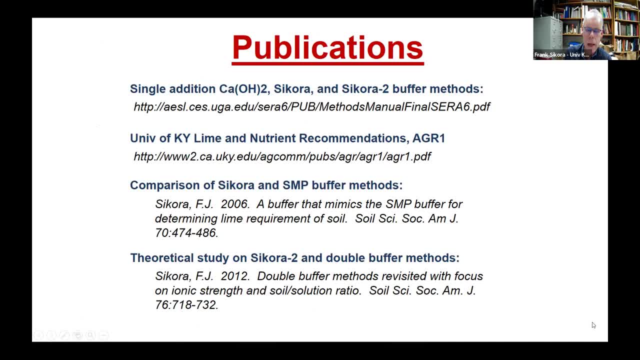 so with that, I'll uh open it up to any questions or discussions you all may have. please, people, jump in. I think this was a great presentation. I I find it interesting that uh three is the magic number for the correction factor, no matter whether whether the soils 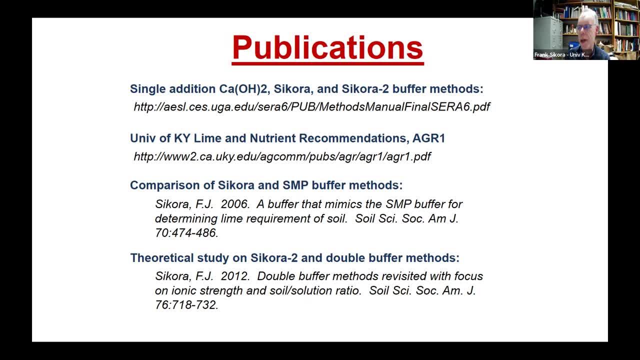 came from three different states, so go ahead. I was real impressed with that. yeah, hey, Frank, this is Ralph from uh Florida. great question: uh say uh, is there any uh ionic strength issue with AE buffer that we have to deal with if we ever working with AE for the same thing on AE? I don't know. I, I didn't look at AE. 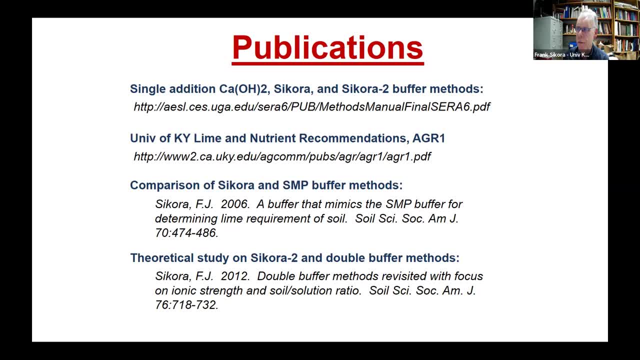 buffer with respect to determining a lime response curve, like with the initial pH. uh, so I I didn't explore that with the AE buffer. I just looked at creating, creating the same buffer pH and tell you through by I'm forgetting what the initial or what the ionic strength is in the AE. 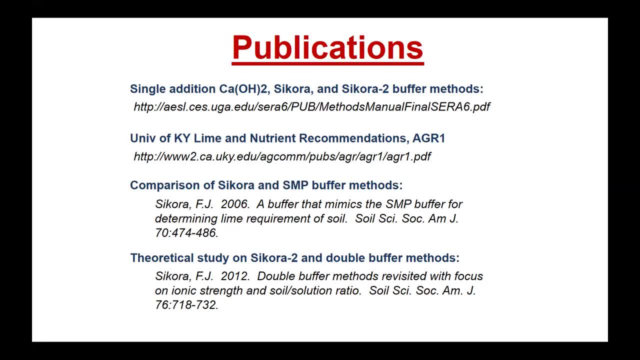 buffer? yeah, that's what I was wondering too, but uh, you know, I know you have added KCL here, but uh, I don't know if anything similar happens with AE2. hey, Frank, this is Brian Hopkins. um, I just wanted you to, not a question, but just uh comment that um, Sakura is actually got a little bit better precision than SMP when. 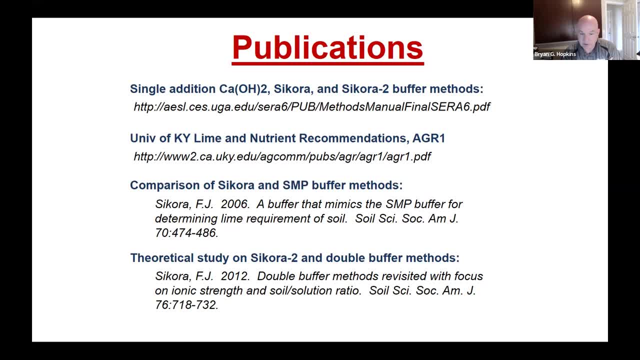 we measure that across Laboratories. anyway, it came out really that and Woodruff came out to on top in terms of precision. so I thought I thought I'd just mention that to you, happy to share that information. yeah, thanks, I, I didn't know that. um, hey, Frank, I have maybe a a little bit of an esoteric question. uh, I noted on the Shoemaker, uh, 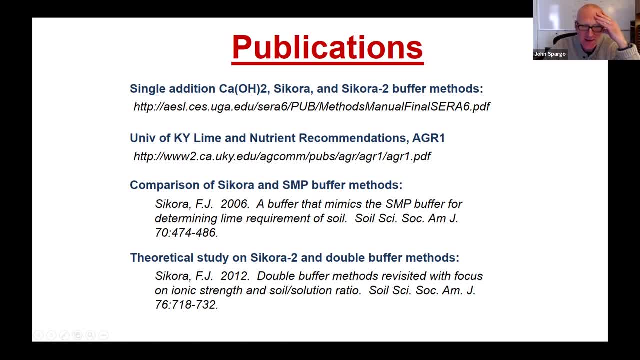 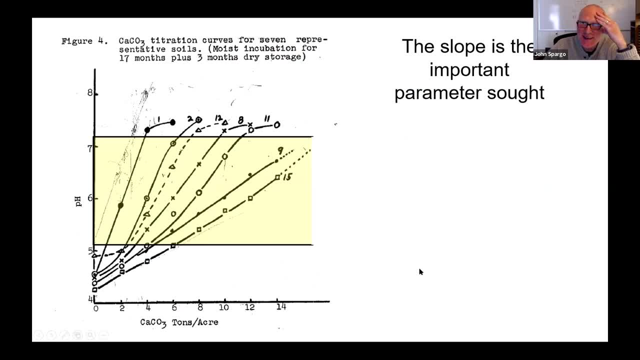 incubation- figure caption: the. the swills were incubated for 17 months and then aged for three. what do you think? what do you think the purpose of dry aging for three months was? I don't know. seems like I, more than just like you know- a random afterthought when we got around to it. yeah, 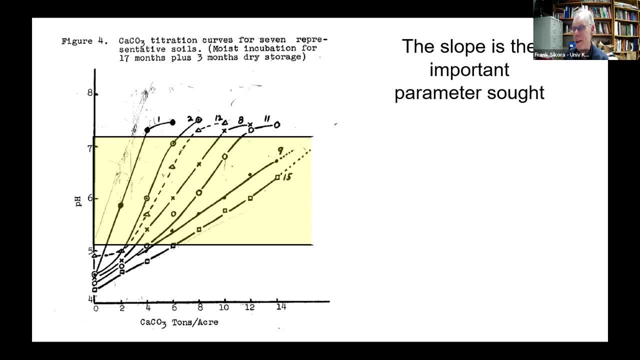 maybe that's how long it took them to get around to it and they put it in there. I, I tell you that thesis has it. there's a lot that is hard to really understand why they did things. uh, but yeah, I don't have an answer, John, I'm not sure. interesting, perhaps. perhaps the student was still. 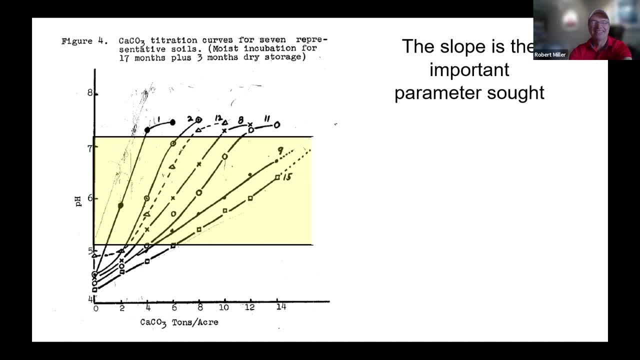 taking classes that semester and he had to put him on this story until he could get to him. so hey, Frank. so I have another question. so I understand the Linearity between where the aluminum takes effect in p871, 72. but but what do you think about these really strongly acid soils? 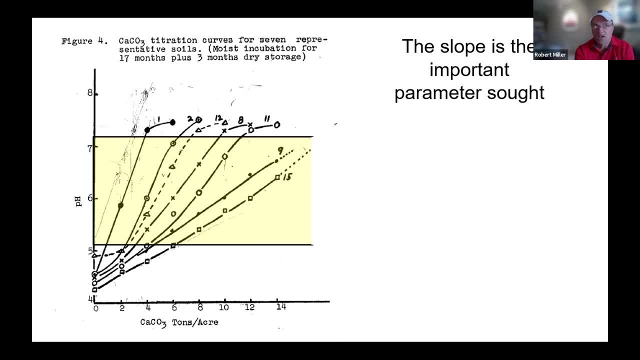 because when I look at databases, I see a lot of these congenital uh Kız cylinder hand, many of these hand moment um uh defense structure instead of a backshell in estouced only I see a lot of soils now that are well not a lot. 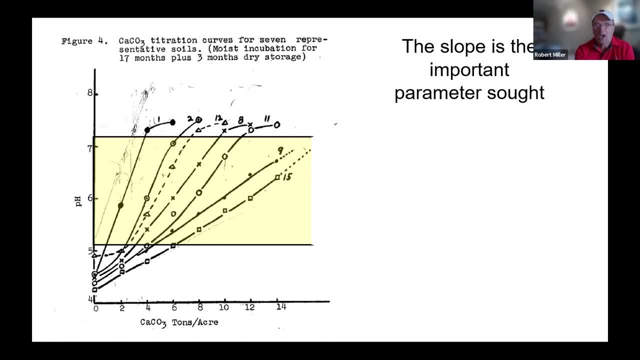 but a significant percentage of soils that fall below that. you know, say, a water pH of 5.4, which probably has aluminum in it. What do you think about down in that area there? Yeah, if they're really strongly acid, you know. 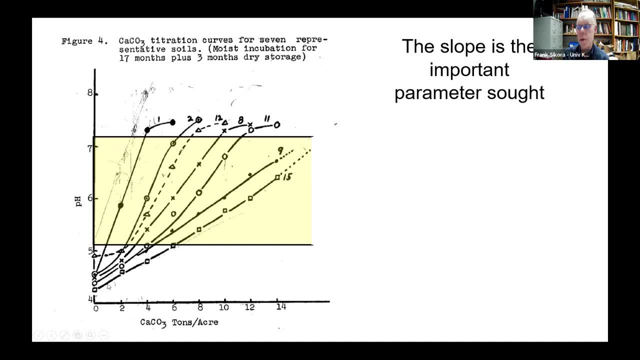 maybe they're still linear down here. You see, some of these soils have linearity, You know, I don't know. I guess you'd have to look at them individually to see what the response looks like in this region below 5.2 or above 5.2. So correct me if I'm wrong. So if I'm dealing with a water pH of 5.4, where I see the aluminum start to be an issue, so one normal KCL pH, that's going to be probably about 4.4, 4.2, 4.3?. 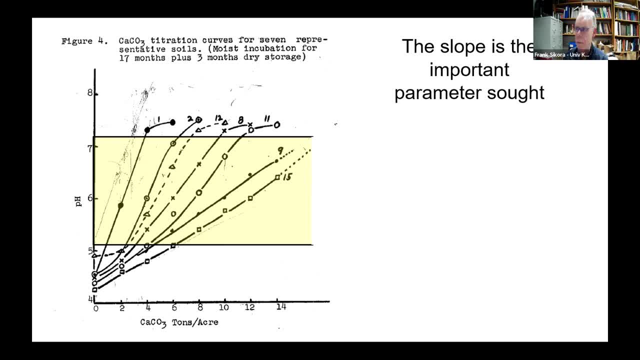 4.4, 5.4.. Yeah, it's about one pH unit. Lower pH is about one pH unit difference. As you increase pH, it's 0.9.. Okay, At higher pH, the difference. And that's what's really confusing in this work. 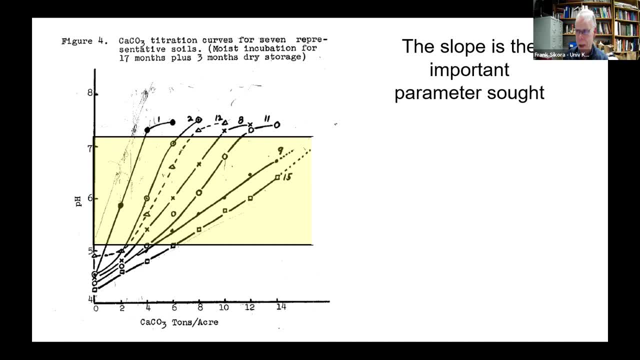 I mean, it's constantly. what pH am I looking at? You know just when I'm looking at my own data. you know, is it KCL pH, water pH It? just it gets mind-boggling sometimes. trying to tease this out, 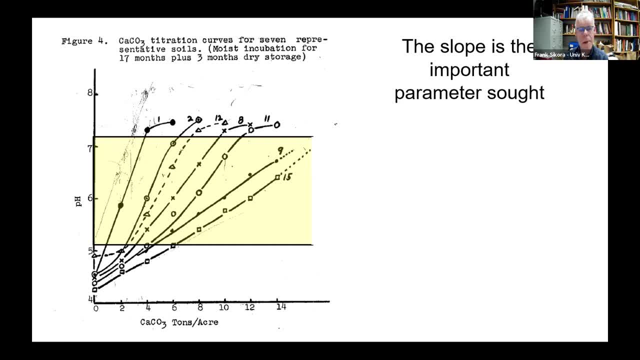 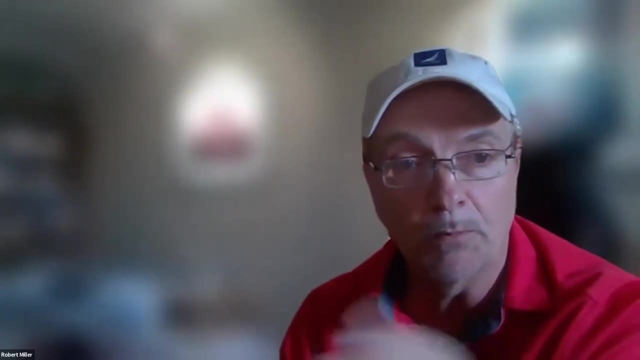 Well, we have time for one more question and then we're going to move on to John Spargo and Sarah Lyons' presentation. Any more questions? Okay, Well, this presentation's been recorded. We can go back up online. The people who are part of the group that's not here today can be more. 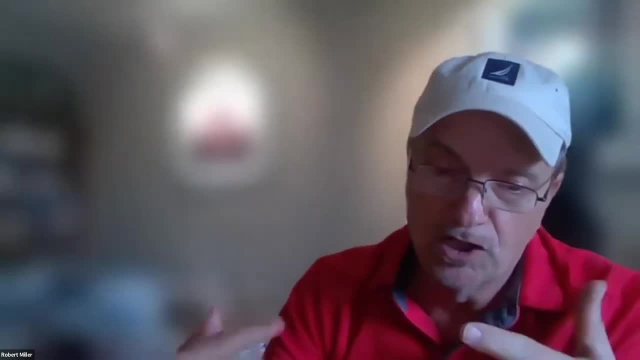 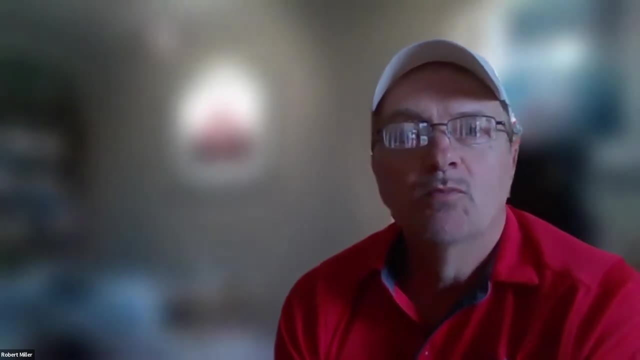 than happy to go there and view this. I think this is a nice, you know dovetails well with what David Hardy did, you know, last month, talking about the pH method. So let's move on. So, John, are you or Sarah who's going to do the presentation on this? 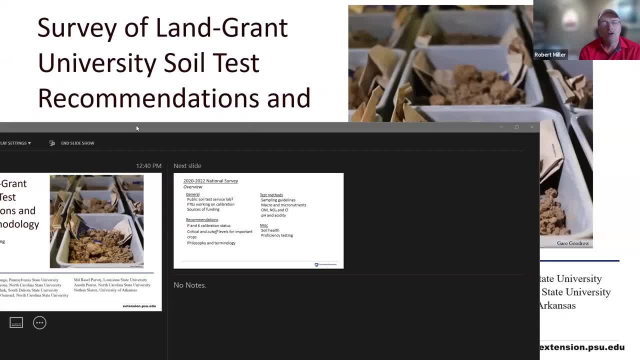 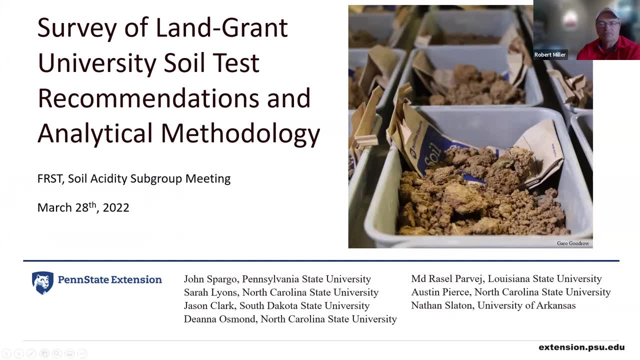 Okay, John's got his hand up. You got the forum. you got the screen sharing. we're set. You're muted. John, Can you see my speaker notes or the presentation? I see the presentation. I think everybody's got the same. 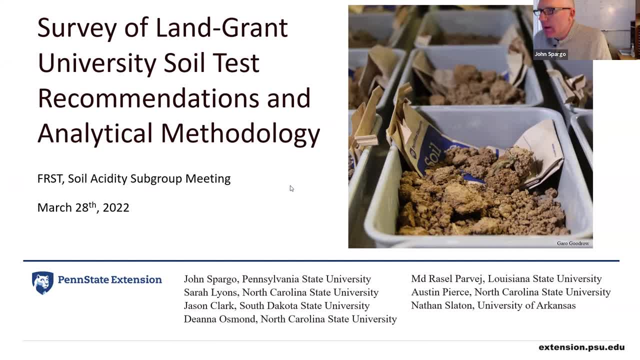 Okay, good, All right, thanks, Bob. So I'm going to try and keep this relatively brief. Got time for additional discussion and to keep us within the hour, Bob, I'm going to go back to you, Okay. So Bob asked about a month ago now if we could share some results, specifically. 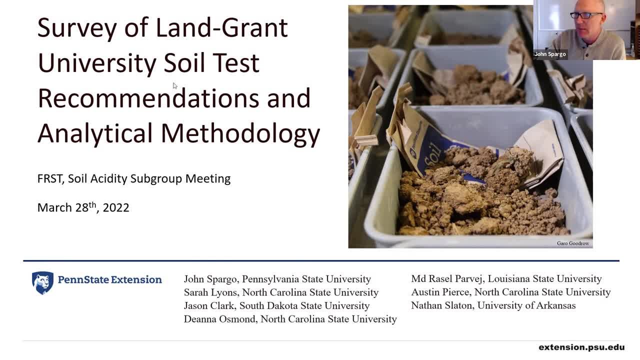 about pH and buffer pH methods that we collected from this survey of land-grant universities. I think most of you have either or both, heard us present, you know, summaries of this survey and or presented, I'm sorry, participated in the survey itself. 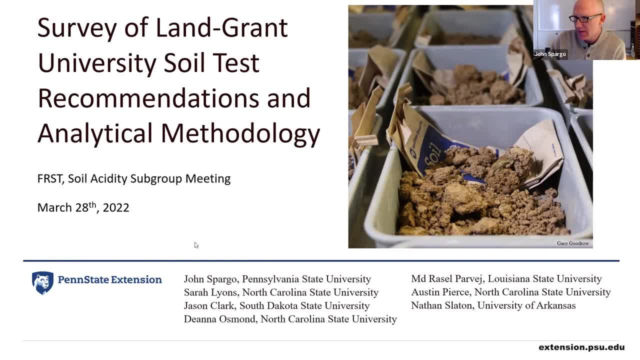 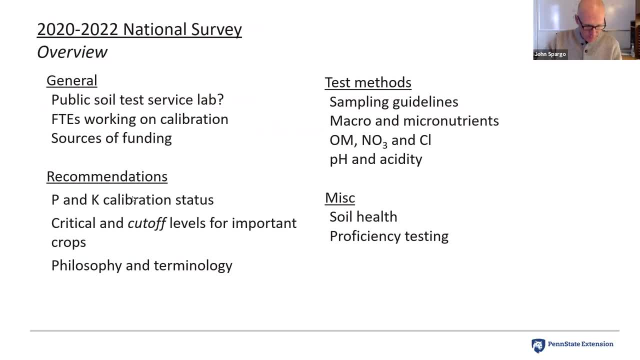 So, hopefully, the stuff that I'm going to share with you today is, you know, something a little bit new. I do just want to provide a quick overview for those of you this is the first time you've heard anything about it. 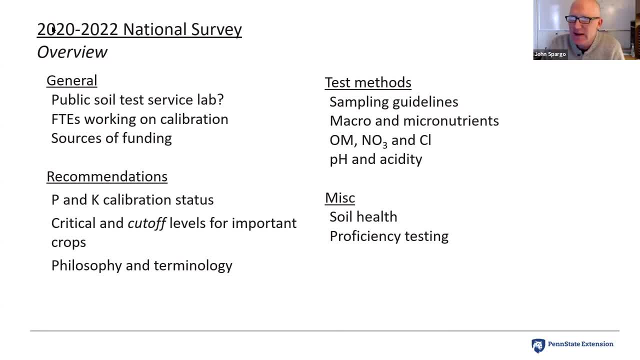 We ran this survey. I think we initially sent it out in 2020.. We've been collecting and correcting and dialing things in for the last couple of years And, as you'll eventually get to see it, because this was a really comprehensive survey- 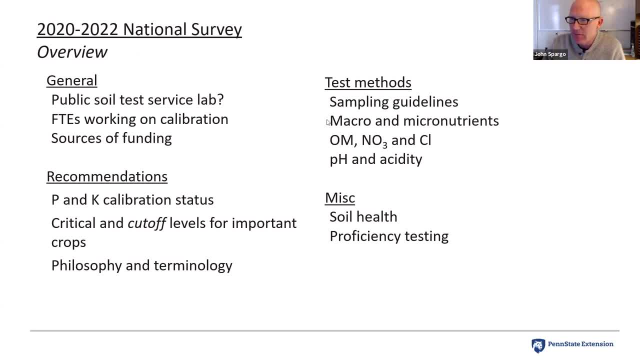 we collected a ton of information and you know everything from general studies. you know a lot of stuff about. you know. does your institution have a public soil test service lab? you know a number of FTEs working in soil fertility calibrations through recommendations. 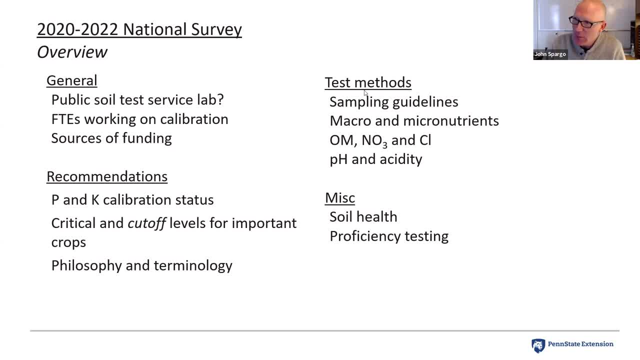 philosophies and terminology. And then we dialed in on soil test methods and you know, obviously today we're going to really focus on pH and soil acidity, but we also collected information on some other things. you know whether or not, if you have a lab, if we're participating in proficiency testing, soil health, et cetera. 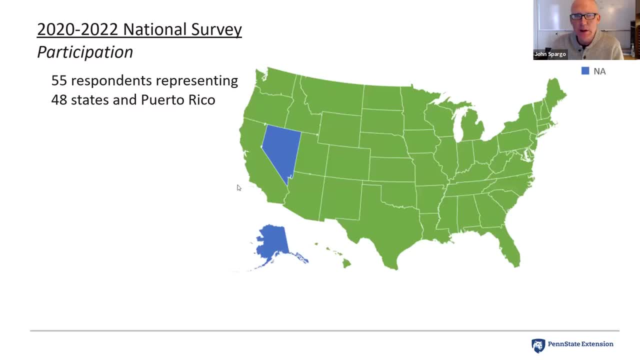 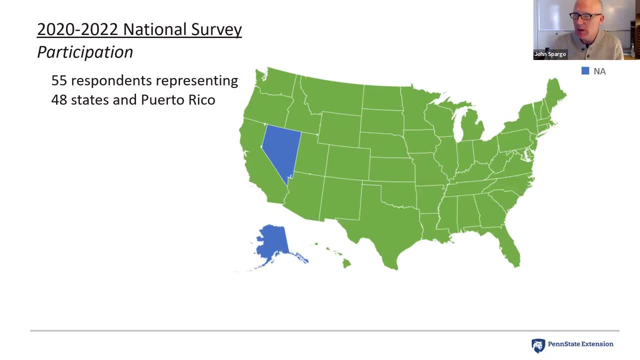 We had really good participation in this and you know, in large part that's because we've got a lot of really good colleagues in this area, as well as the leadership. We distributed these through each of the regional coordinating committees and sort of tasked the chairs with really riding herd on this. 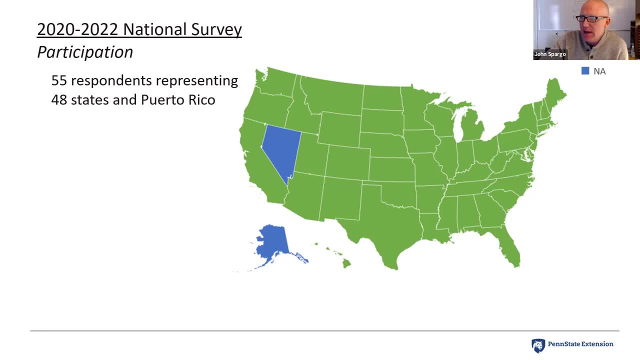 and making sure we got responses from as many states as we could. In the end, we ended up with a response from every state: 48 states plus Puerto Rico. We only ended up missing Alaska and Nevada And, no surprise, neither one of those has a soil fertility specialist to answer these. So 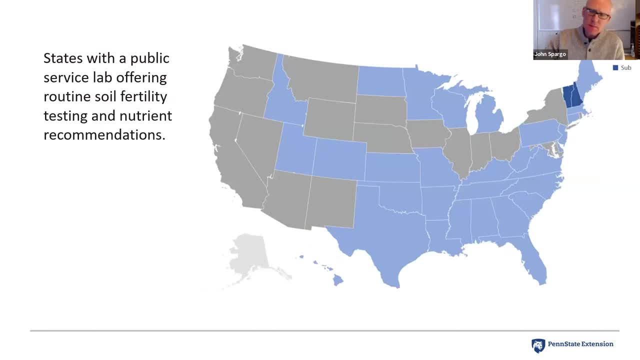 the other thing. I just want to share this one piece with you. You know we were asking a lot in addition to you know the types of soil, fertility research and about recommendations. we were asking a lot about methods And you know, one of the things that we recognized is: 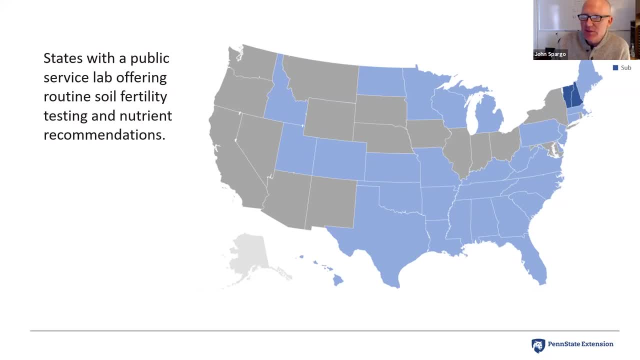 that, whether a state does or doesn't have, you know a service lab, you know has implications for not only how we view, you know our recommendations, but also you know the view or engagement and you know the analytical methods themselves. So at the time of running the 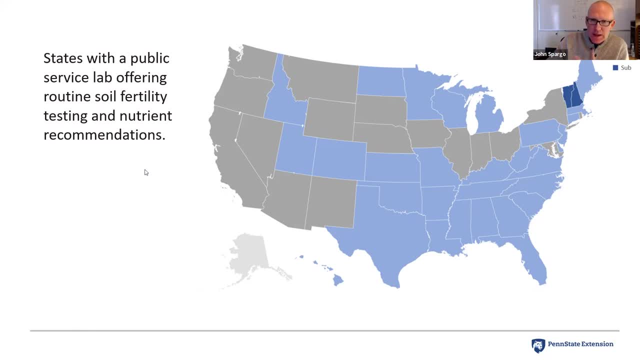 survey out. these are the 30 states where there currently is, you know, a public survey of 30 states And we're asking a lot about methods And one of the things that we service- lab offering soil fertility testing and nutrient recommendations. 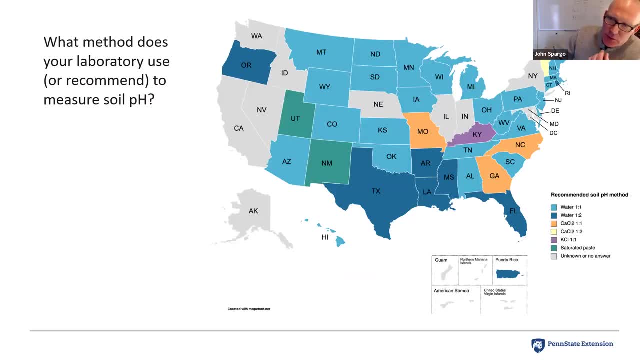 Jumping right into methods with regard to soil acidity, we did ask a number of questions about, you know, how folks were measuring pH and or buffer pH, how they were making lime recommendations. We've got some additional details And I just want to note that you know we did ask about things. 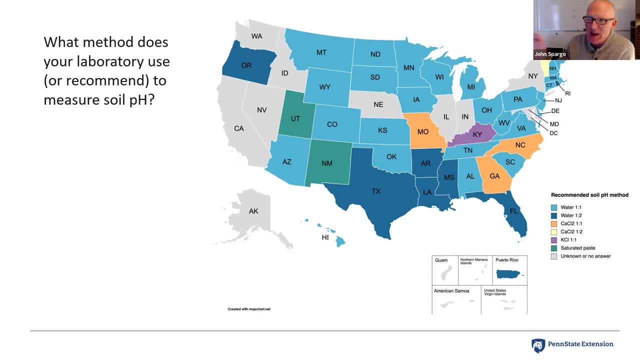 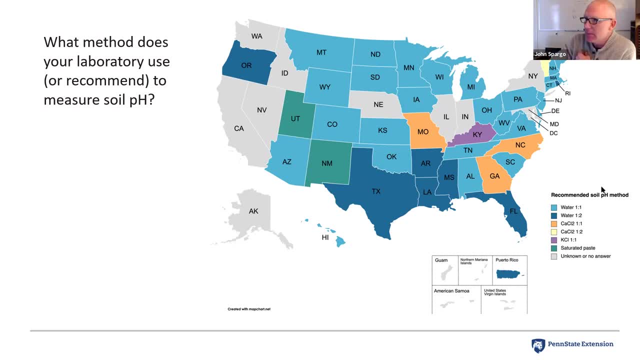 taking the deeper dive. So first, looking at pH methods, you know the dominant one is clearly pH and water one to one. We do have a handful of southern states that are using the wider ratio of one to two And I think there's probably pretty good explanations for that. Just a handful. 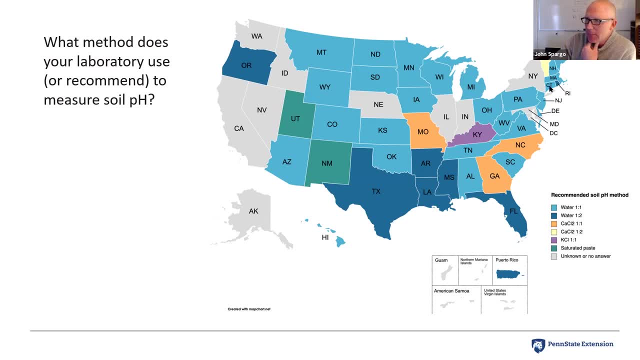 and a hundredth molar calcium chloride, And then again at the one to one. Vermont's method was dialed in for a one to two, And I'm not sure what the divergence was on that one. Just an interesting note. Of course, Kentucky the outlier. one molar KCL And then a couple of 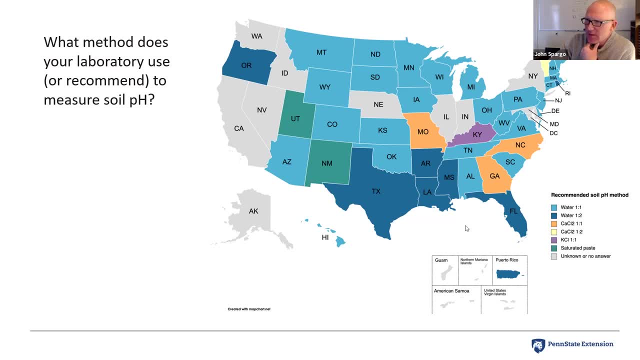 the western states, where they're recommending a saturated pH. So one note just to circle back and put things in context. here we asked the question: does your laboratory or if you don't have a laboratory, do you recommend using this method for measuring pH? Looking at buffer pH, I think I've 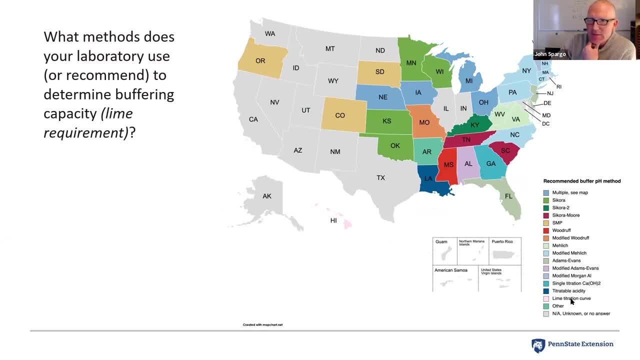 got an accurate count of 14 different methods. Obviously, some of these we may be splitting hairs, We might be able to bend together malic and modified malic And, you know, from what we just learned in the last 30 minutes, maybe the Sikora and SMP. I did not realize how the 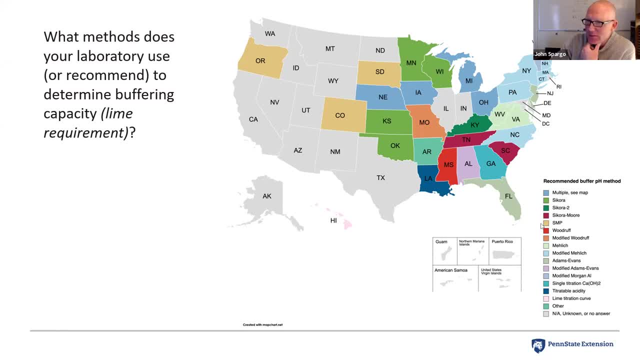 Sikora 2 diverged from these two And that was. yeah, I learned a lot in 30 minutes there. Thanks for that, Frank. A couple of, I think, interesting notes here. Vermont never really used a buffer to make their lime recommendation, So they're not going to be using that. They're not going to be. 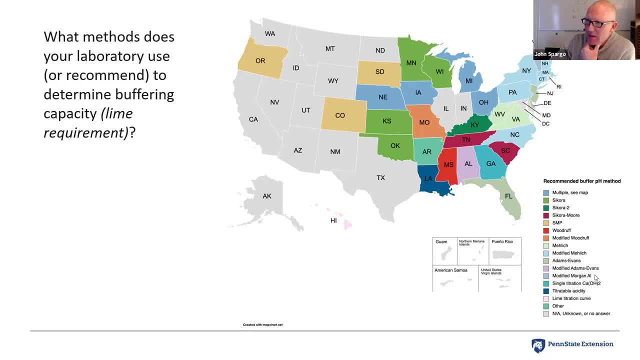 using that. They're actually using extractable modified Morgan, extractable aluminum to get an estimate of soil buffering capacity, And I think Frank mentioned you know the method they use in Georgia with you know the single titration point: calcium hydroxide. 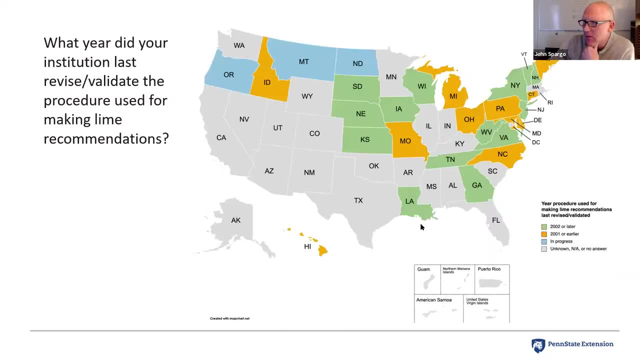 Just a few more notes I think are relevant to this discussion. One of the things we also asked is: what year is the last time that the lime recommendations, or procedures for making lime recommendations were revisited? And then we just, Sarah, pulled these maps together and just split it into three bins. 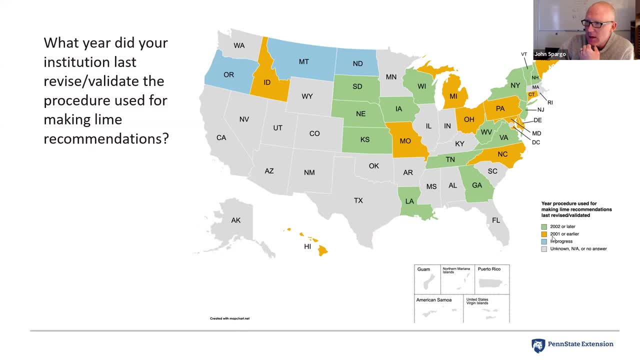 Since 2002, so within the last 20 years, more than 20 years ago or before 2001- are currently in progress And I was really pleased, you know, seeing this summarized this way. You know, 14 of the states responded. 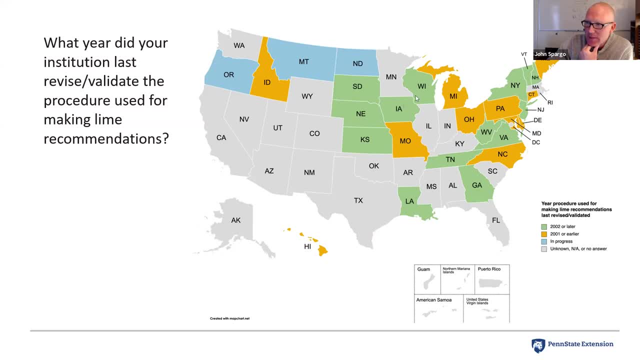 You know, noted that they've looked at this within the last, within the last 20 years, 10, it's been, you know, more than 20.. Three currently in progress: You know Western states where soil acidity is starting to become an issue. 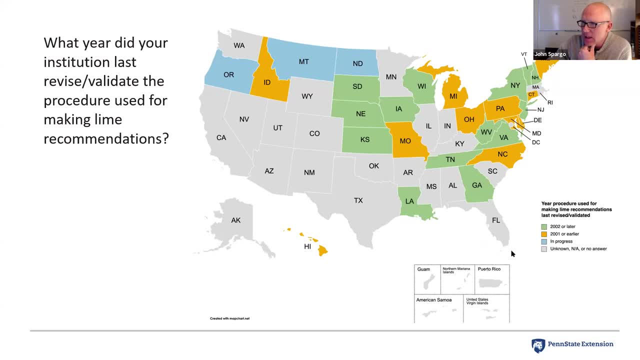 And a little bit disheartening, but you know, not calling anybody out- is that in this- you know, these gray boxes- includes nine states that weren't sure what the provenance of their lime recommendations were, And I think that's a good thing to keep in mind. 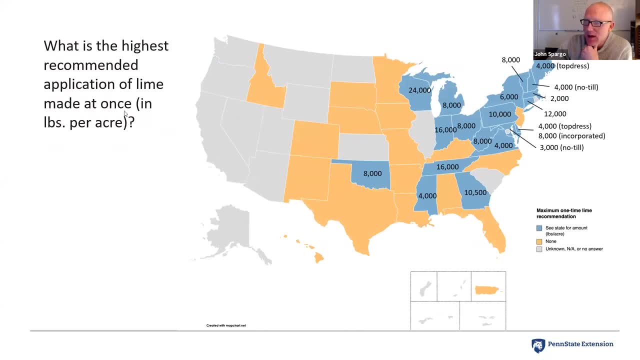 And I think that's a good thing to keep in mind. Frank mentioned you know, Frank mentioned you know many states cap their lime recommendations at a certain threshold. That was one of the things we asked about. So these in blue have some ceiling limit. you know the maximum amount of lime that they would recommend being put out in one application. And it ranges everywhere, from, you know, two times or 4,000 pounds all the way up to 24,000 pounds. And it ranges everywhere, from, you know, two times or 4,000 pounds all the way up to 24,000 pounds. 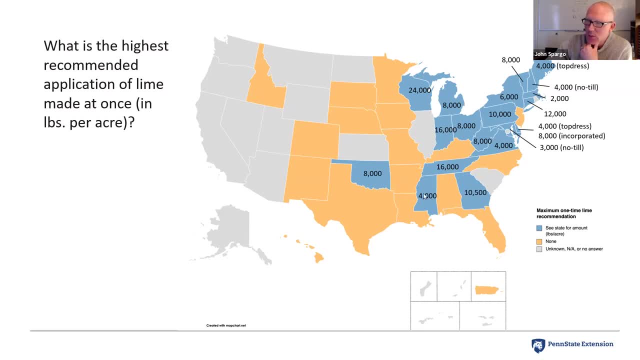 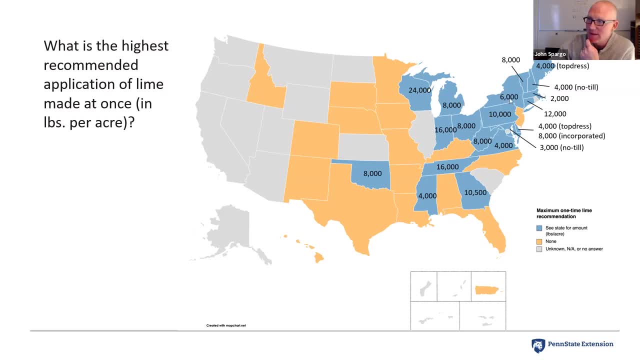 I know, specifically for Pennsylvania, this is not 10,000 pounds of calcium carbonate equivalents, That's 10,000 pounds of actual material. So if we give you a lime recommendation, you know say of you know 5,000 pounds of calcium carbonate equivalents, but you're going to work with a material that's only 50% calcium carbonate equivalents, well then, that's going to meet your cap. We're not going to recommend applying any more than that. 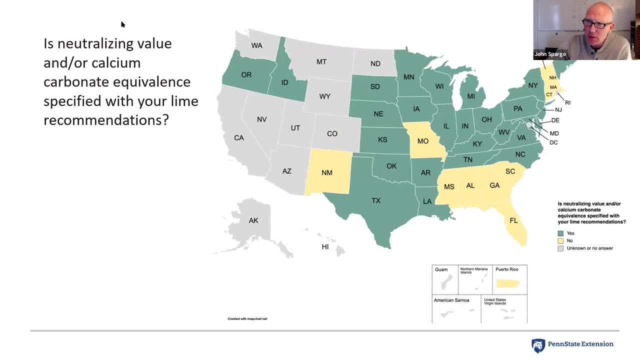 Finally, leading into the next question, do you specify either neutralizing value or calcium carbonate equivalents with your lime recommendation? And most states do responded that they did. There are a handful that don't. And you know this kind of gets into some of the other discussions and nuance and you know the survey that Bob sent out last week, late last week and you know sort of trying to get a handle on what the 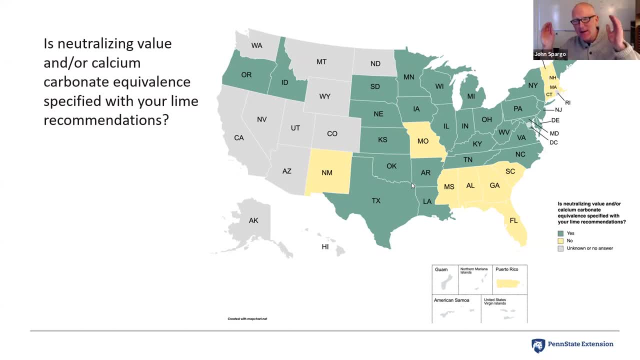 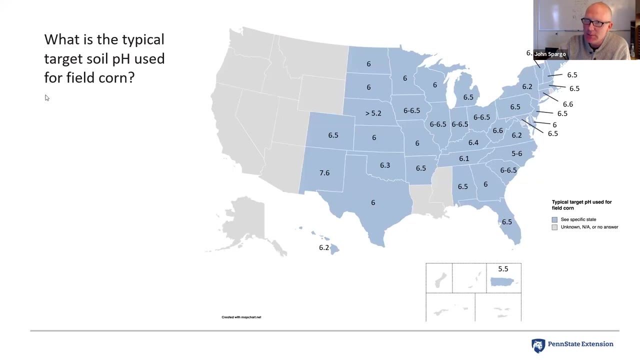 how we come up with our lime recommendations and sort of pulling that, that the calcium carbonate equivalents, out of that, so that we can, you know, normalize things across recommendation systems. And finally, we asked what the typical target pH is used for field corn And you know most states are coming in somewhere between 6 and 6.5,. a few notable outliers: Nebraska, as long as we're over 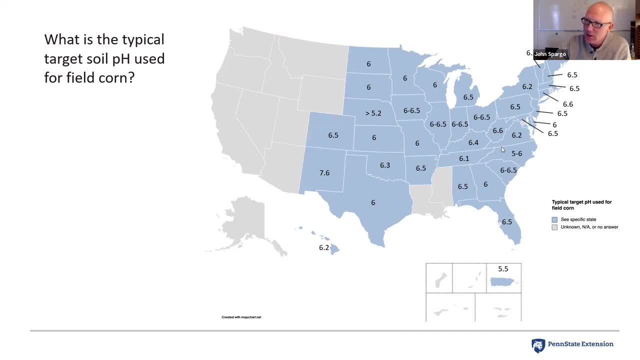 5.2, everything's good. North Carolina, for mineral soils, has a target pH of 6,, while for the organic soils, you know, 5 or close to 5. But in general between 6 and 6.5.. 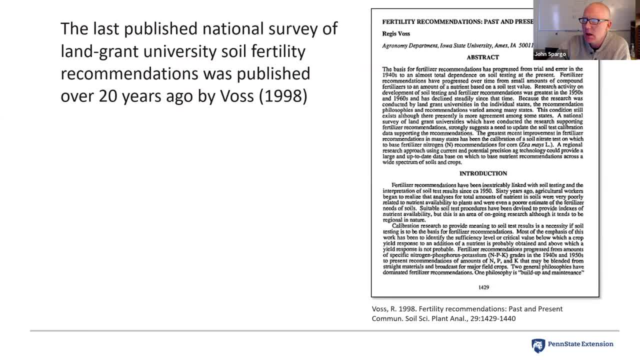 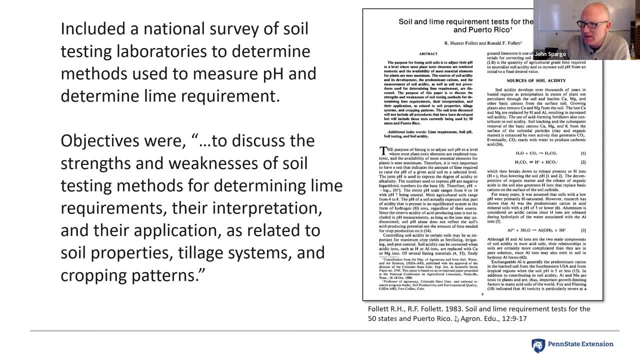 And I'm going to quickly share a reference If you guys haven't seen this paper: Follett and Follett from 1983, a really interesting paper, a really interesting paper published in the Journal of Agronomic Education, A just a really nice overview, sort of extension version of you know, soil chemistry- I'm sorry, soil acidity, the chemistry of soil acidity. 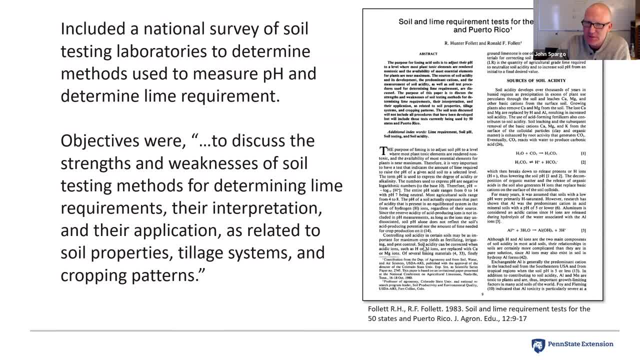 But they also did a pretty extensive survey of labs in different states and they weren't clear whether or not it was university labs or all labs. But they also did a pretty extensive survey of labs in different states and they weren't clear whether or not it was university labs or all labs. 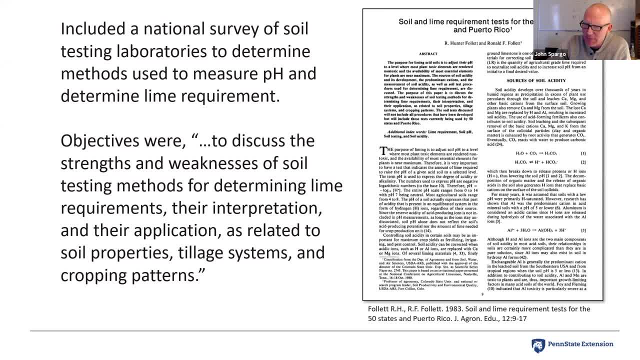 But got a good, a really good summary of methods used to measure pH as well as buffering capacity, And then did a really nice sort of strengths and weaknesses of each of the different approaches. A really nice paper and, I think, relevant to our discussion here. 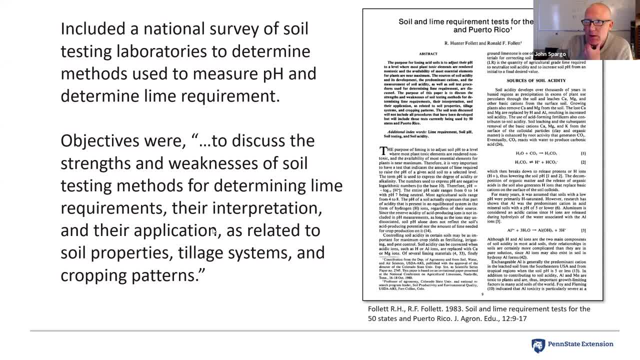 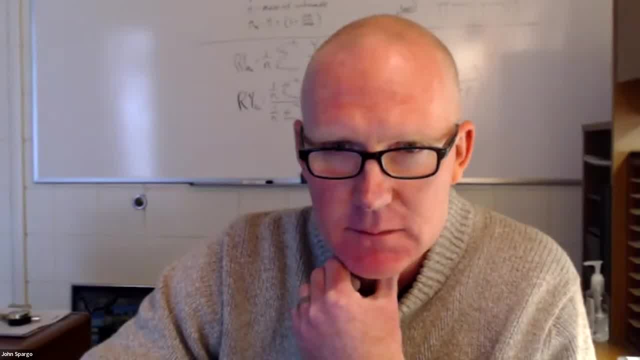 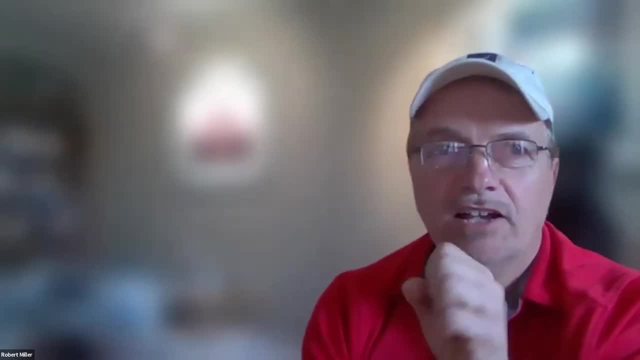 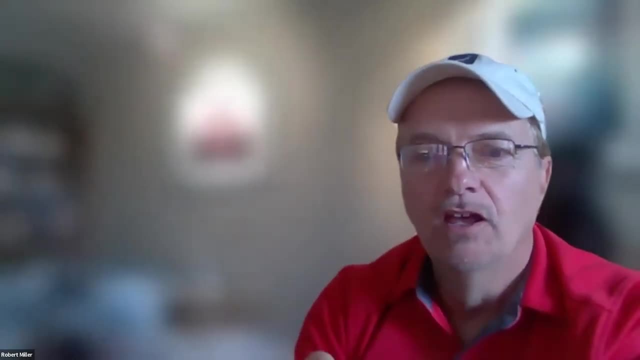 And I'm going to cap it off there And invite questions or comments. so, john, i think you did an excellent job of kind of piecing together the ph methods, the buffer ph methods, but i think it's really important to see both the target ph people are going for and then 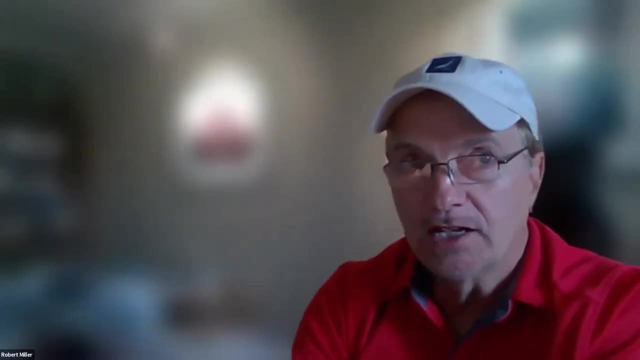 what they max out the line and i think to make a valid point that we're not talking about tons of lime, we're talking about tons of material that can go on the field. you know, it's quite shocking. it looks like a lot of those were about 8 000- 10 000 pounds was kind of the upper limit. several. 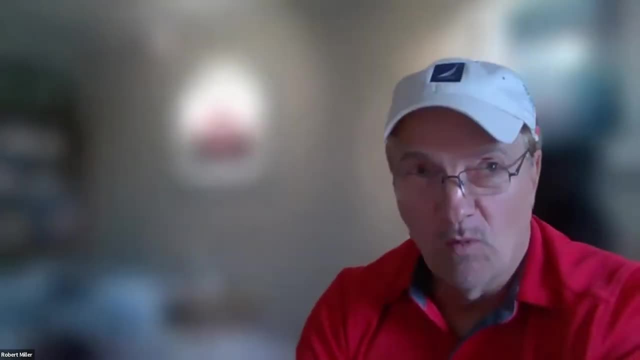 at 4 000. i'd like to understand why somebody had 24 000 in there. i, i, i. if they have plot data to say that 24 000 where they had a very acid soil, that'd be great, but i, i, that's more of a curiosity. 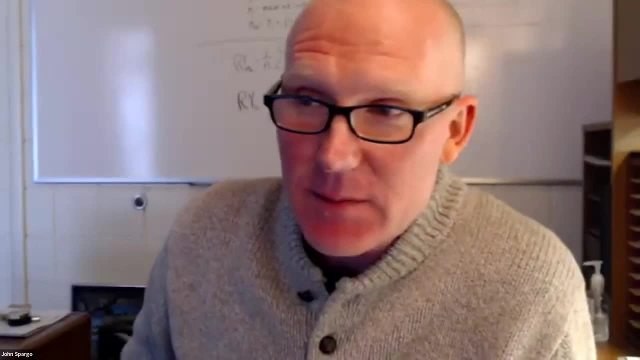 more than anything. so i mean, we, we've got some soils that you know are buffeted, are that acidic, and and we come up with a lime recommendation. you know, you know, we've got some soils that you know are buffeted, are that acidic, and and we come up with a. 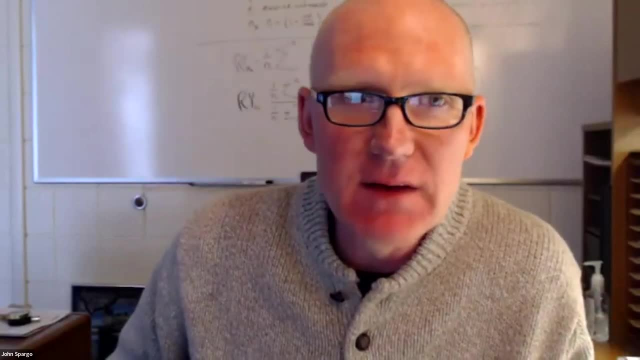 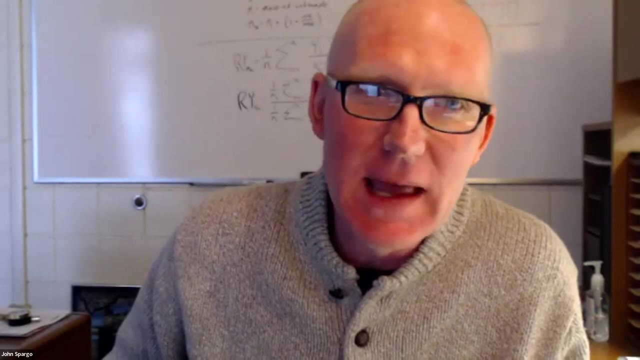 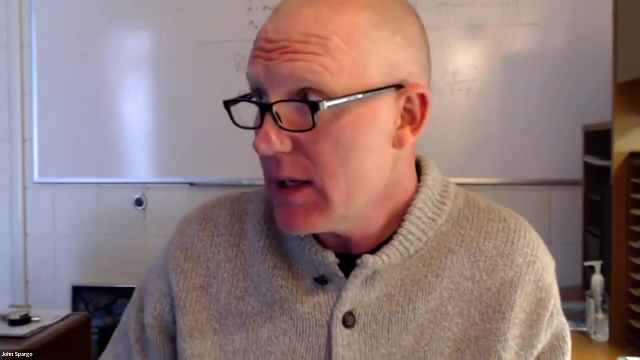 penciling it out. it would take, you know, 20, 25, 000 pounds of lime to hit a target ph of six, five um. but it, you know, comes back to economics and or logistics. it just doesn't make any sense to put on more than, uh, you know, 10, 000 pounds of material in one shot. where we end up in in a real pickle is 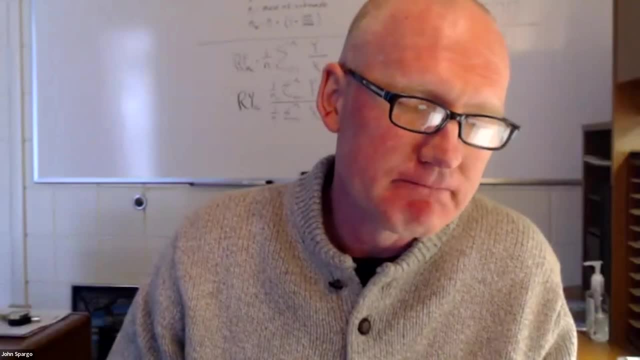 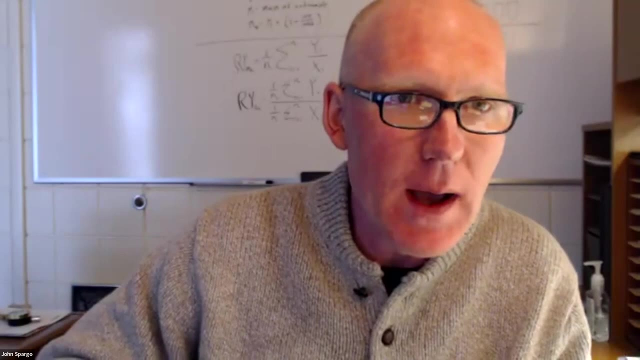 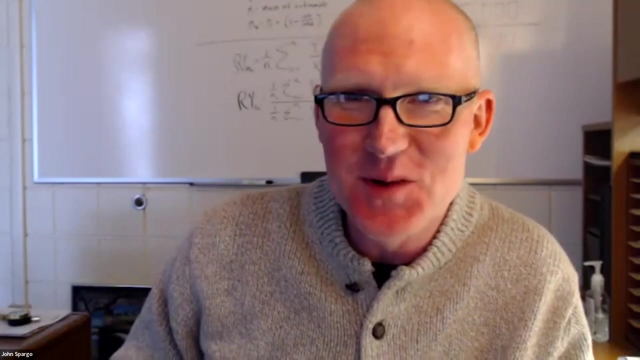 uh, especially in, uh, you know, like you know now getting away from, from agronomic production, thinking about, uh, you know a right-of-way or, uh, you know mainland reclamation kind of thing, where you know it's, it's. we're not talking about managing this, this. you know this piece of ground. over several years we've got one. 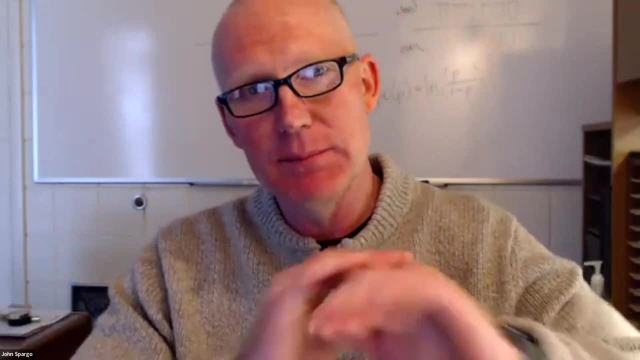 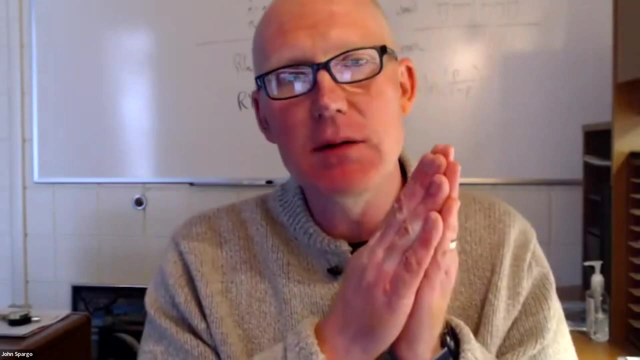 opportunity to get in with the bulldozer, apply this material, get it incorporated and get it planted. um, and you know what we've worked with those folks on is, you know if, if you can't split it out, separate it out over time, um, you know you got to separate it out by, uh, field operations. so 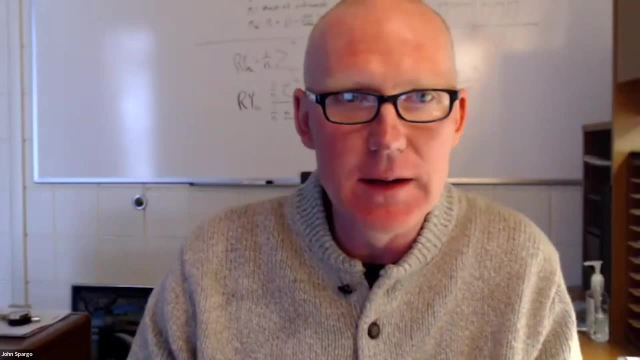 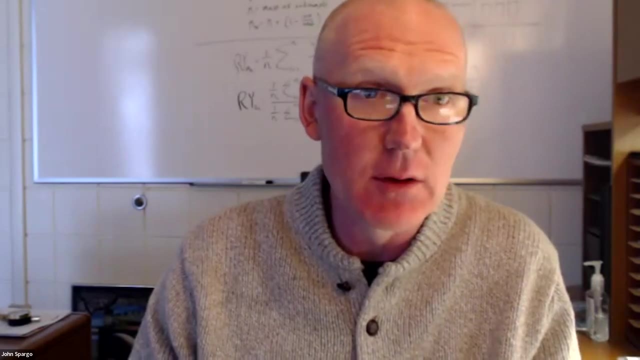 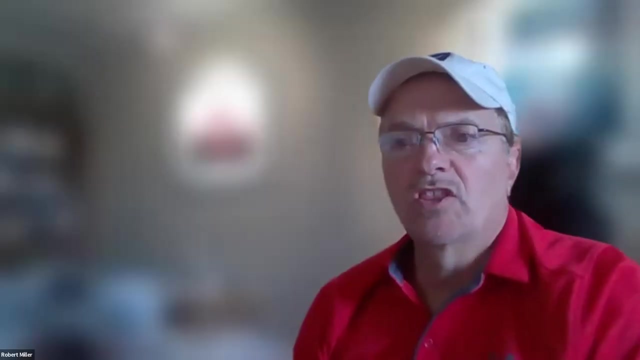 you know, maybe we put, you know five tons down and, and you know, run it in with a moldboard plow and then you put another five tons in and hit it with a really aggressive set of discs and just try and get it as well incorporated as possible. yeah, that's, that's one of the challenges, excuse me. 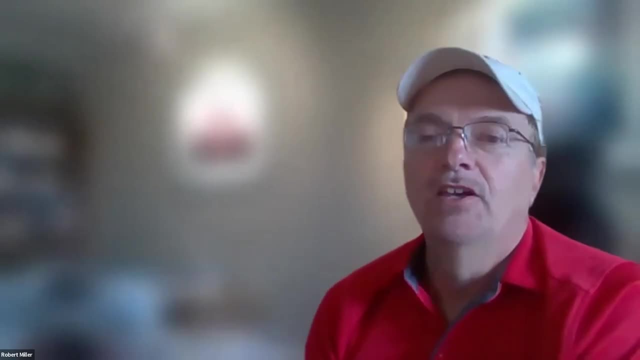 that i've read into you, where you get into these no-till systems and the guys you know. absolutely not i do not want tillage out there. and yet you know i've seen several fields where the subsoils are in the threading threshold of four, nine to five one and you kind of go: well, you've got some issues there developing. 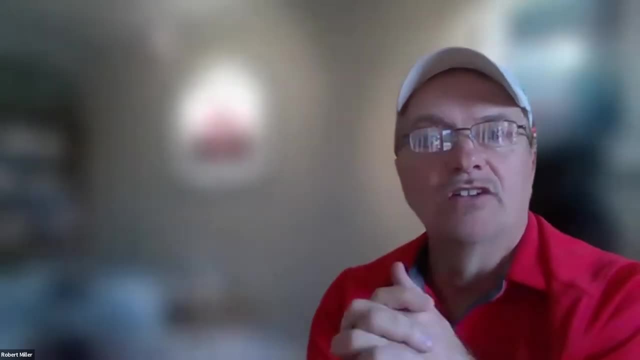 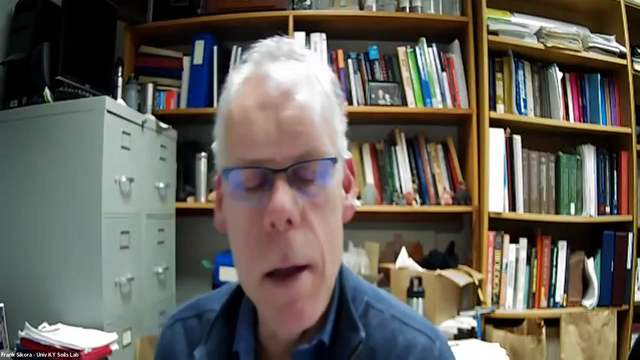 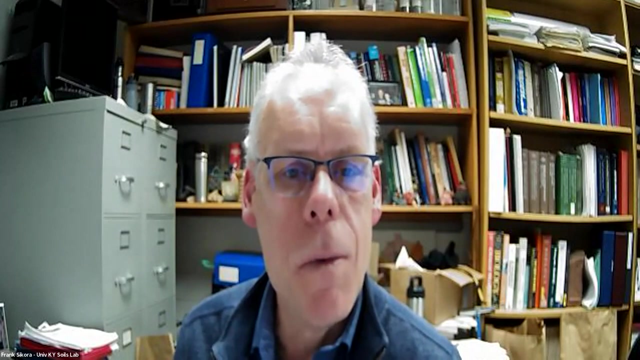 over time, especially from long-term use of an hydrous fertilizers. so any other questions. i'm surprised nebraska ph for corn is anything at 5.2 or greater. is that due to lack of lime in nebraska or why is such a low ph for corn in nebraska? you know, go ahead, john, if you have any. questions about that. yeah, i mean i can speculate. uh, i i think you know, if you look at where you know, aluminum doesn't start to become toxic until you hit 5-2. if i the real question, i think frank, is: uh, why are we liming all of our other soils to 6-5? you know it doesn't. corn doesn't need it. the. problem is that the soybeans or the alfalfa, or you know the other crops in the rotation, do, um, and they, they did a bunch of work in virginia. um, you know, way, way, uh, north carolina too. yeah, they don't require such a high ph. yeah, they, they, you. 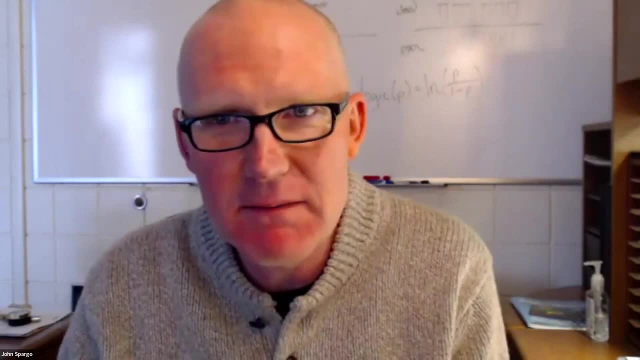 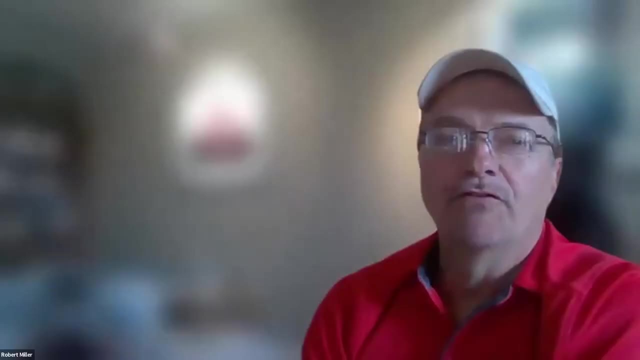 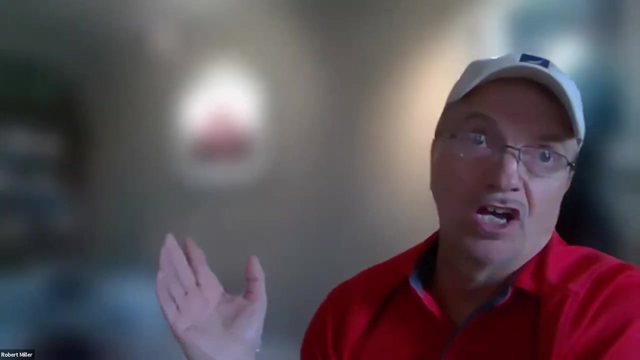 know corn, corn yields topped out. you know five, five, it's fun to your point. frank about, excuse me, brian, uh, frank to your point about, uh, nebraska. there's a lot of lime sources in eastern third of nebraska. you know the first uh seven, two counties, eight counties in from the missouri river. there's a lot of lime deposits there. the. 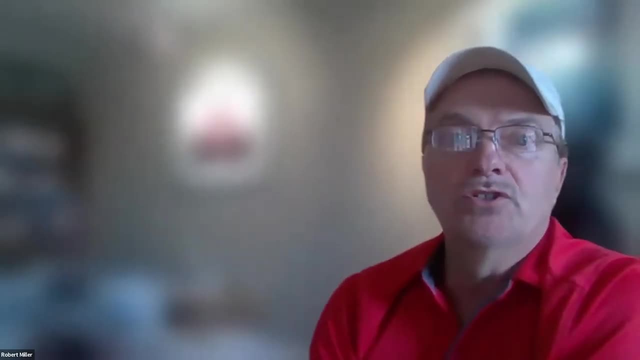 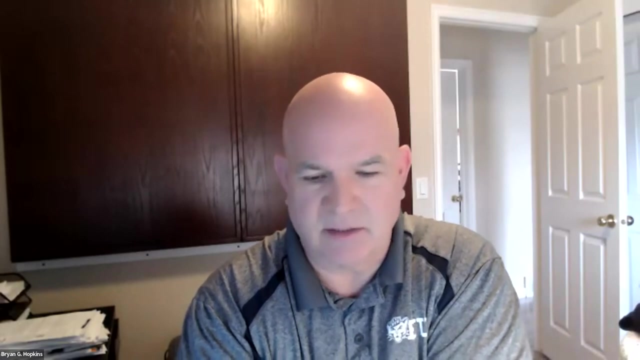 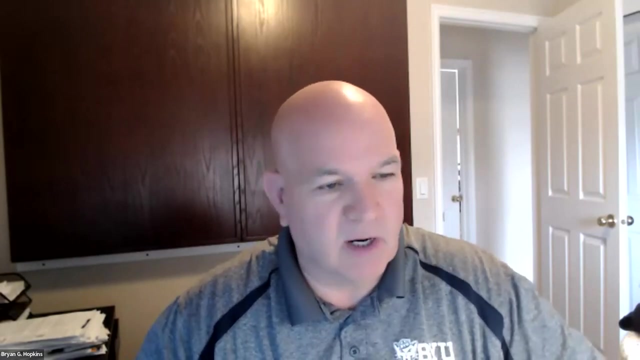 problem is is, once you go beyond that, the trucking cost becomes a big issue. i was going to mention that i used to work for servitech manager lab and pasting nebraska and i i wondered that exact same thing. and you know we we consulted when i worked for them. we consulted on about a million acres. 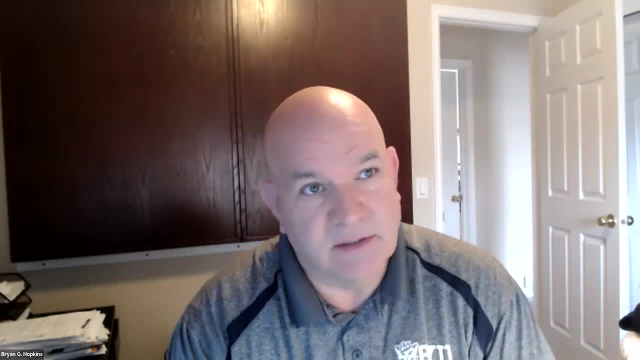 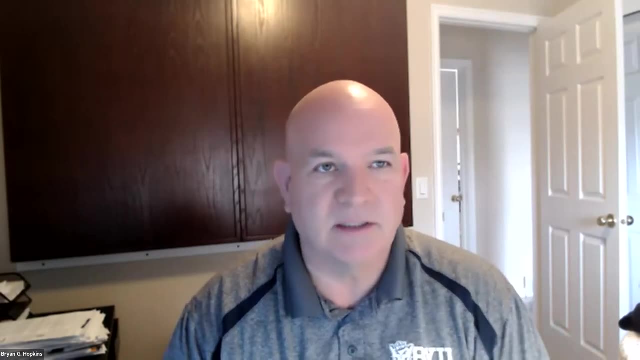 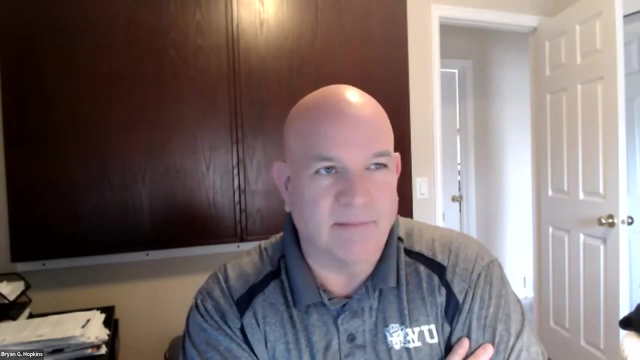 of crop ground and what? what we discovered is that, um, is that a lot of those subsoils, even though the the soils are acidic, The subsoils are still fairly calcareous in a lot of the areas, even in eastern Nebraska, And so we, frankly, you know, oftentimes our guys were just not finding that. 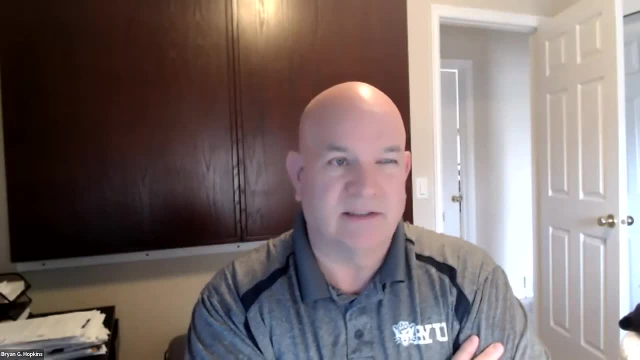 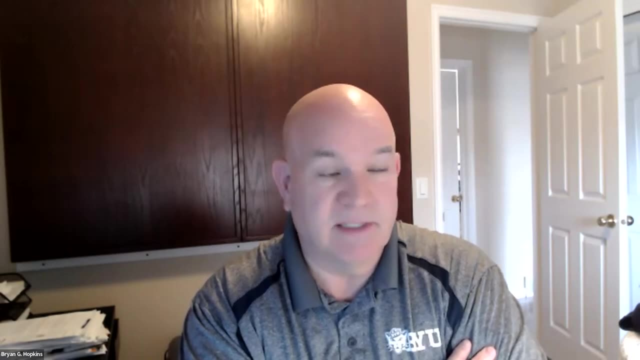 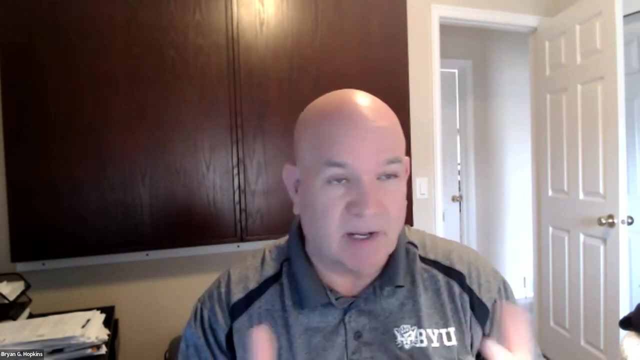 they had to line to a very high level. Now, in some places, though, where the subsoils were more neutral or acidic, we did find that we really did need to bump that up a little higher than that level. So, anyway, that's my opinion is that it's flavored by that subsoil chemistry. 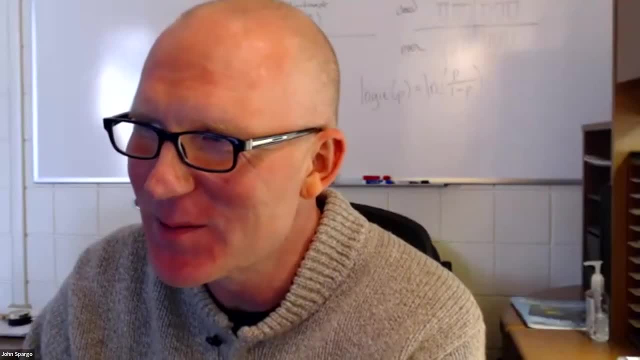 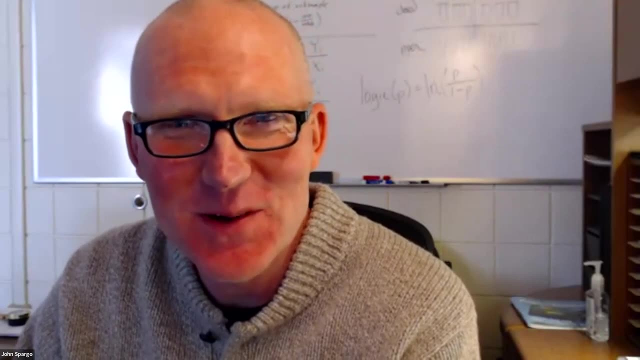 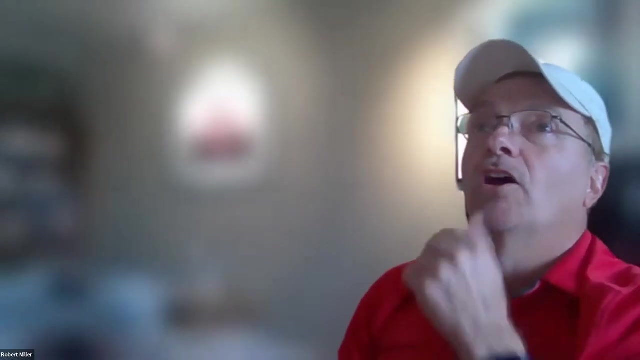 So you know. the other question I've had with those is: what do you do about the triazine herbicides? So continuous corn PHF5, too, Yeah, Yeah, Well, you know, it's just. it's interesting that that. and I don't know if it's a good thing to do, but it's a good thing to do. I don't know if it's a good thing to do, but I don't know if it's a good thing to do. And I don't know if it's a good thing to do, And I don't know if it's a good thing to do. 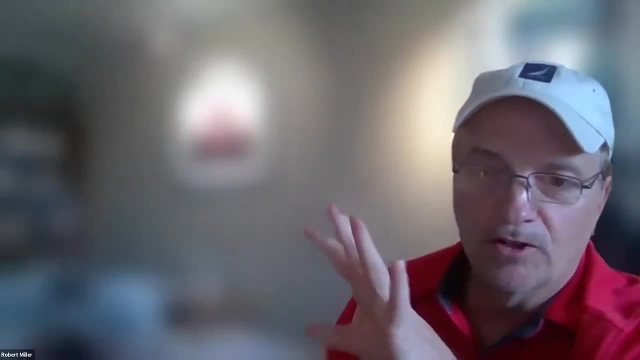 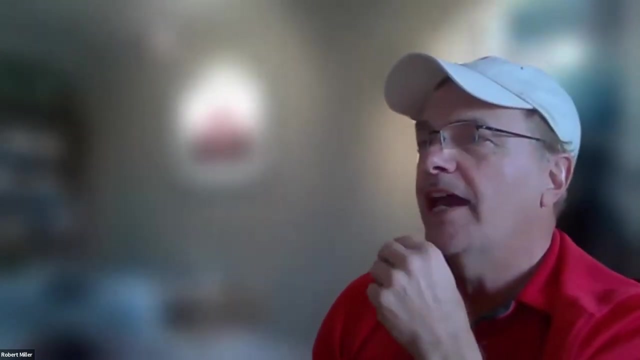 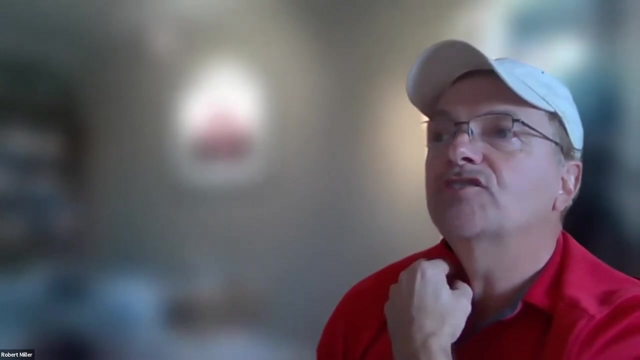 don't disagree with you. I would say liming rates of 6.2 on corn, and the fact is you don't want to go in there very often, so you may push it up a little bit, but whatever, Okay, well, we're coming up here. we've got just a few minutes left, So we've got on my calendar here set for the next. 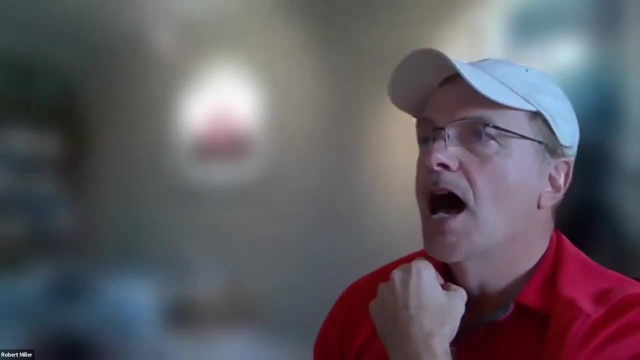 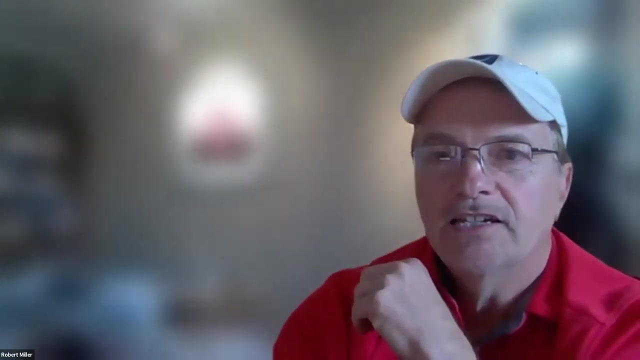 meeting on the 18th of April. So if that all works for everybody, we'll see everybody at 10 am mountain time, noon eastern time on the 18th of April. We're going to have a discussion from one of our colleagues here. Just a second I'm going to move my screen over. Luke Gedabani is. 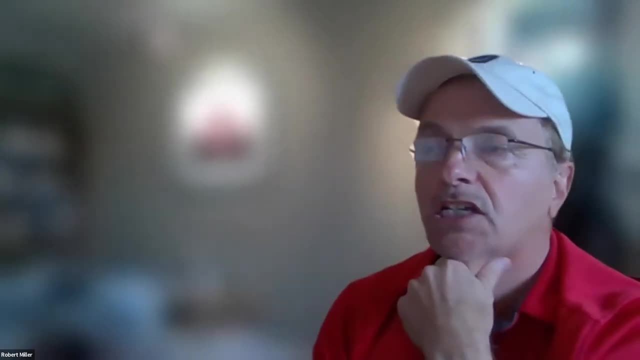 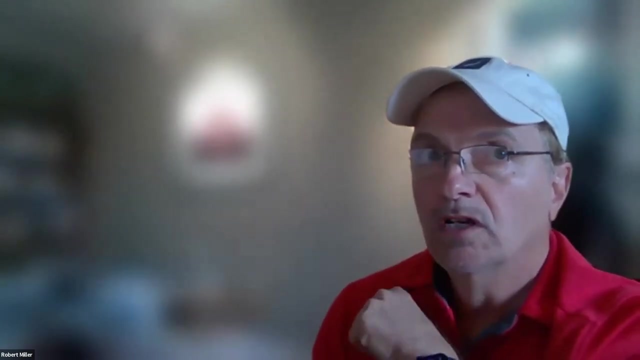 going to do a presentation on soil, the chemistry of soil acidity, and hopefully by then I'll have some data back. I have six respondents on that survey I sent out for coming up with the lime wrecks from the from the various states. I'm going to try. 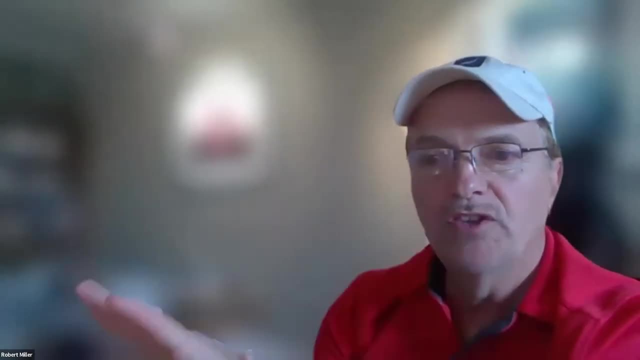 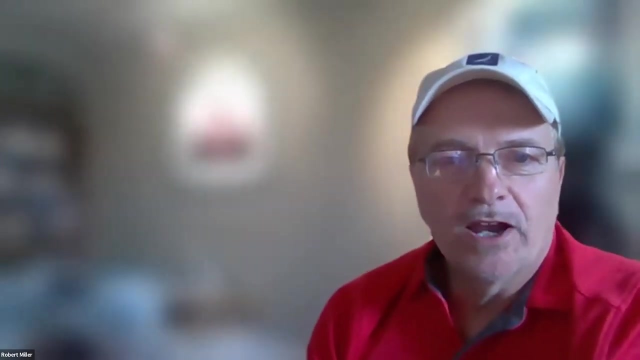 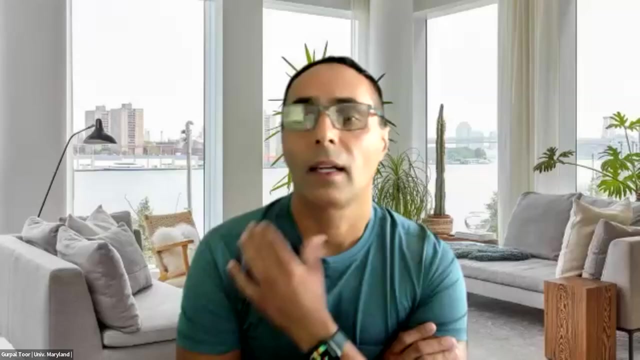 and get that up on a Google Docs area so everybody can just go in there and edit that on that and take care of it rather than returning all those emails. So any other comments before we break this off? Hey Bob and John, I just have another comment and it seems like you know a lot of states are. 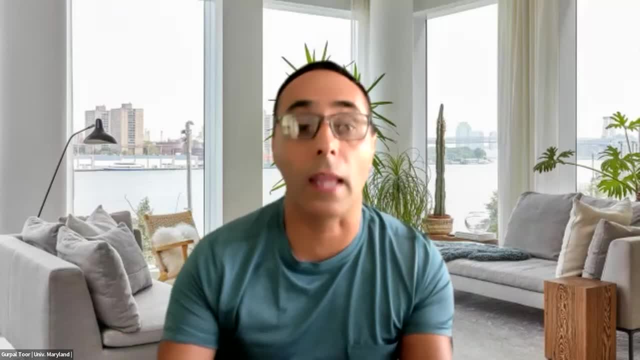 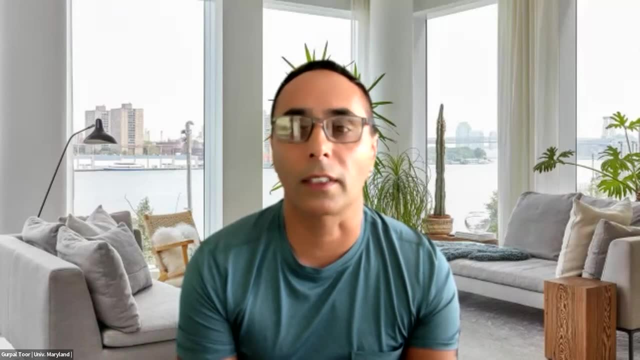 just kind of keeping it to six and there's. if there's not a further gain in anything, Why do we keep adding Like? I think that seems like a really good point to discuss And you know we are in our state. we are thinking of revising our recommendations. If this, is there a real benefit to getting to 6.5?? Can't you just do six and reduce farmer some money that they have to add the lime? We look at it as an investment and you're also going to take care of those low spots in the field that you can't account for when you're soil sampling. There's. a lot of variability and it's an investment. you know it's. you're constantly acidifying your soil With all of the nitrogen, and so you know it's more about get it up to that point and then enter a maintenance level, instead of having to do four or five tons a year. So from a practicality standpoint, 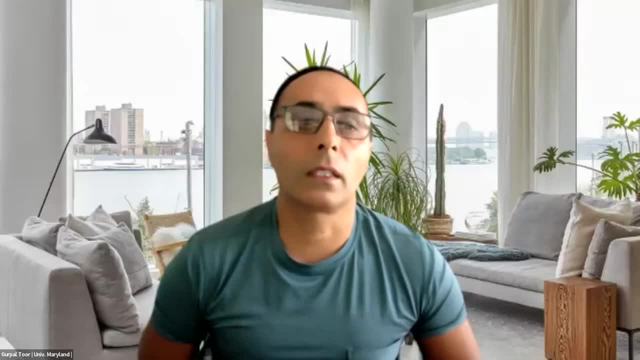 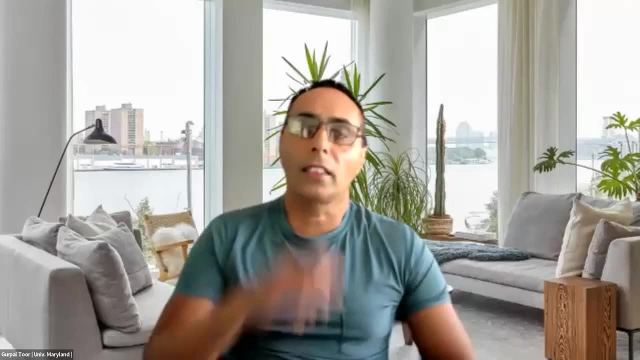 it just makes it easier to manage. Well, I think it's a relevant point that you know some of the legume crops love that little higher amount, right, so go ahead. No, I guess I was saying that, so J's point is good. I think that's a good point. I think that's a good point. I think it's a good point. 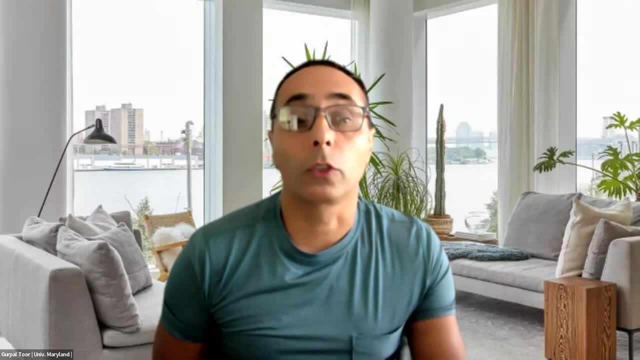 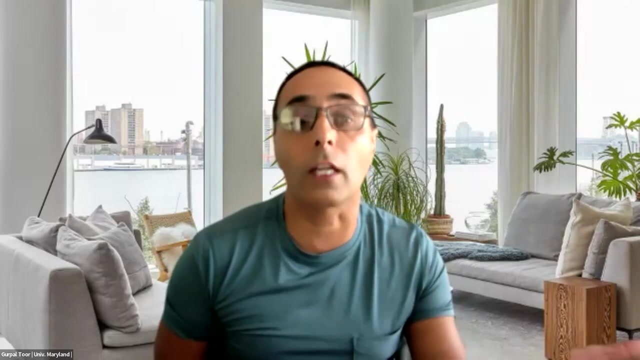 But the challenge is we keep getting rainfall. So even if you add more, it's not going to stay there for much longer, depending on how much rain you got. So I'm not really sure where. like, I follow the logic that you have tremendous variability, but if you captured a really good 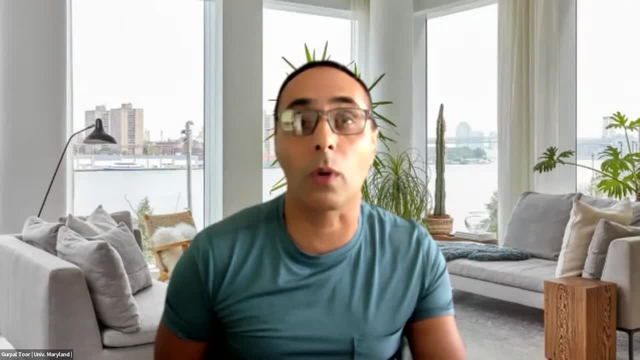 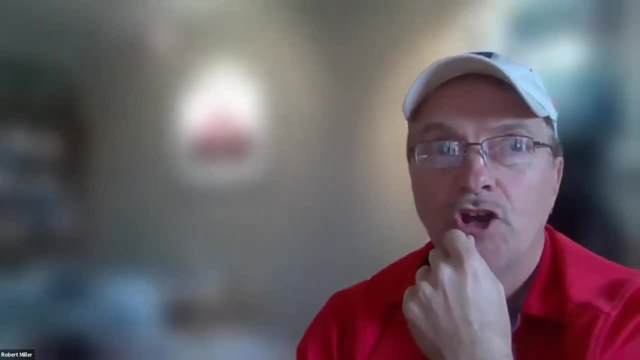 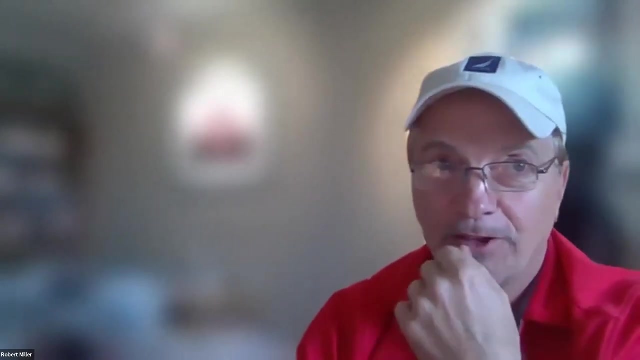 soil sample. that takes care of the variability. maybe you can live with a little less lime application in those fields. Well, and you know, I'll make one addition to what J said. You know the other thing: the applicator isn't perfect either, right? So you know, I don't, I don't know what the precision is on applicators. 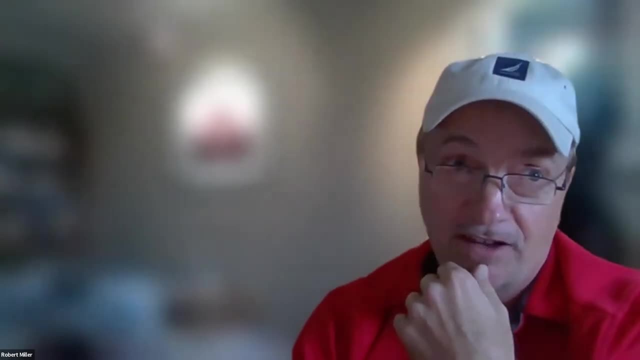 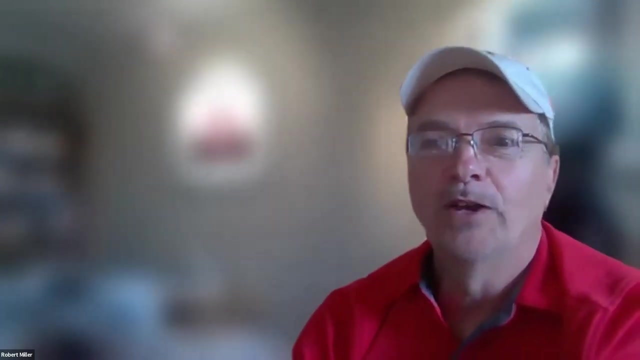 for lime employment. but I would say it's probably easy. several say 200, 300 tons the acre variability. So you got the variability in the sample, the spatial variability and the variability applicator. We kind of put you know- a correction factor in for all that. So Kentucky, we recommend. lime. We recommend lime to get to 6.4, but we don't recommend any lime if it's above 6.2.. So 6.2 is kind of the trigger to whether recommend lime or not. That should probably go down to six. maybe you know We only recommend lime if you're above, if you're below six or not. 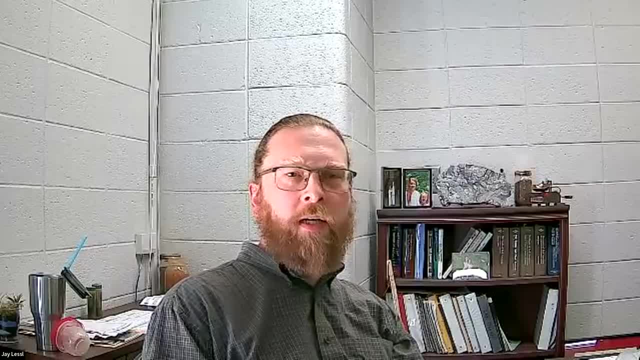 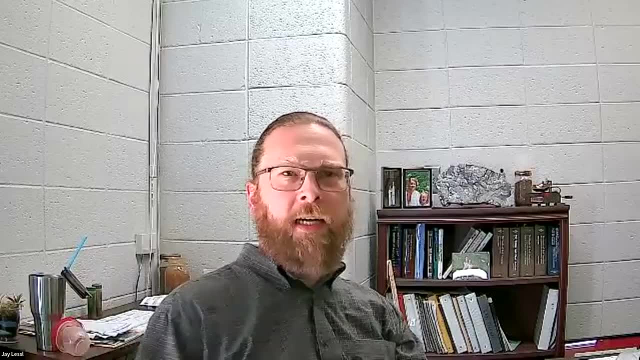 We actually give recommendations for both. So our target is 6.0. but if you we have growers that want to know what you know, if they if lime's cheap that year and they want to try to get it to 6.5, we also.